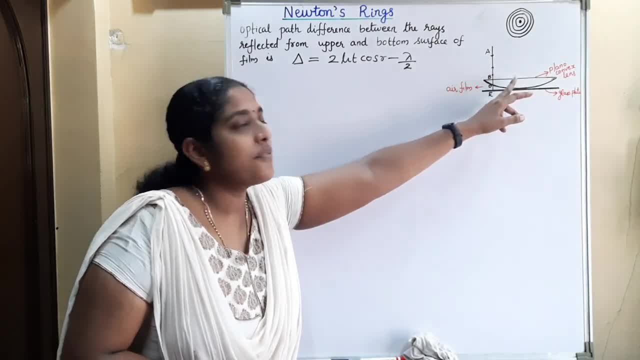 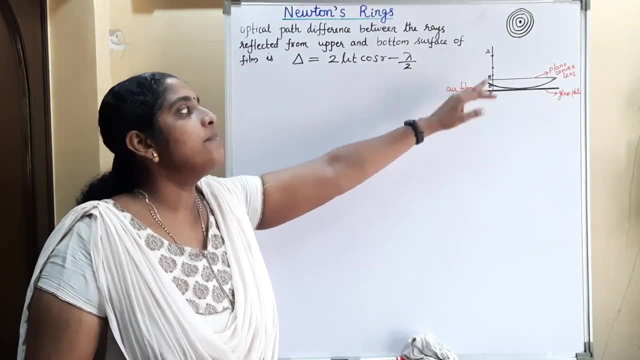 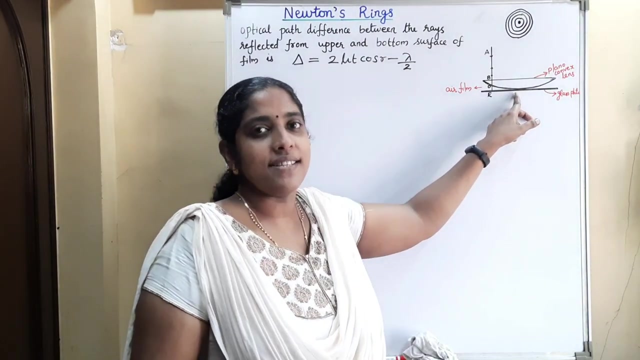 and a glass plate. A plano convex lens of large radius of curvature is placed over a glass plate, Then an air film will form between this lens and this glass plate. The thickness of this air film is zero at the center, and from the center outwards that thickness is 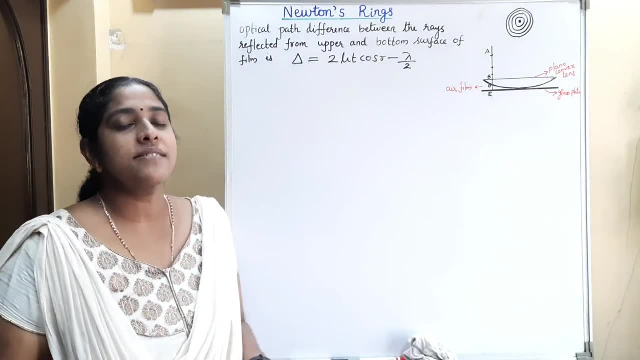 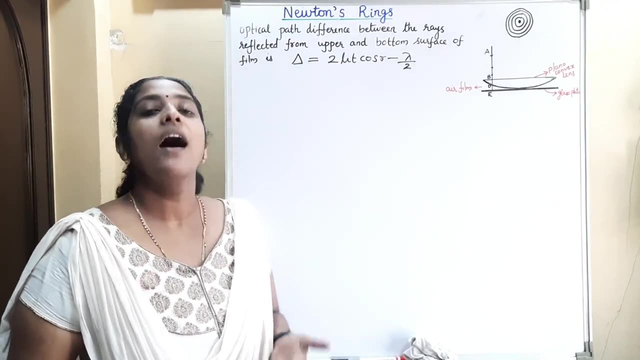 progressively increasing. If such a system is illuminated by a monochromatic source of light, what happens Then? Newton's rings are produced. How Newton's rings are produced Here, when the light is incident on the system, the light is passing through the lens and 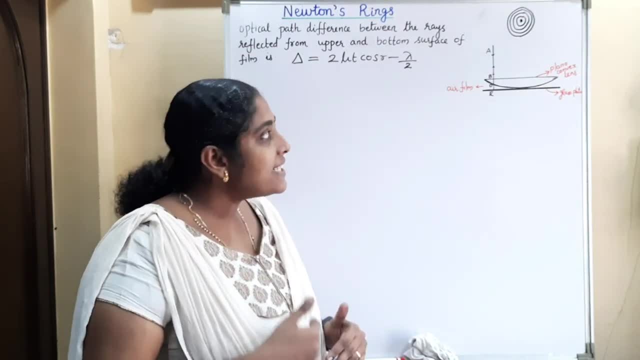 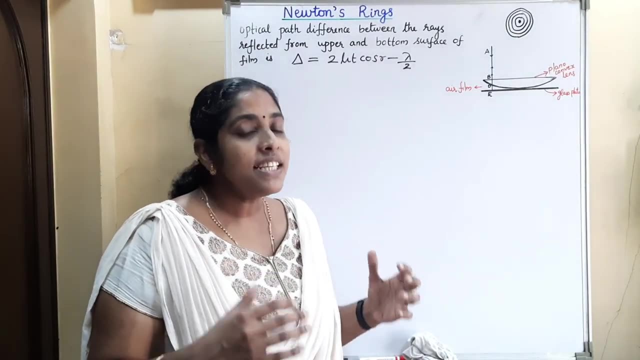 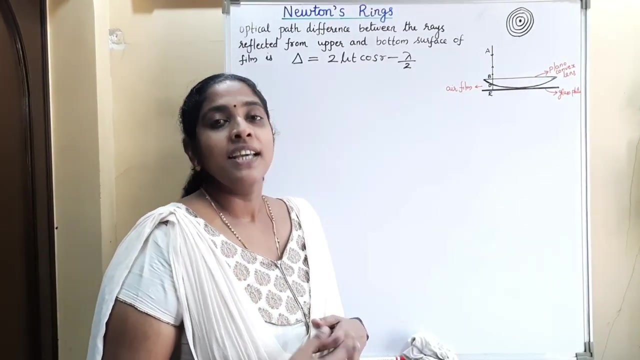 it falls on the air film, Then the light can be reflected from the upper surface of the film and bottom surface of the film. When these two reflected rays will superimpose each other, interference patterns are produced. If such an interference pattern in the reflected 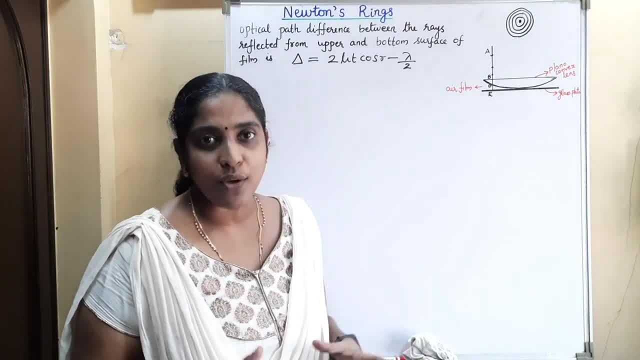 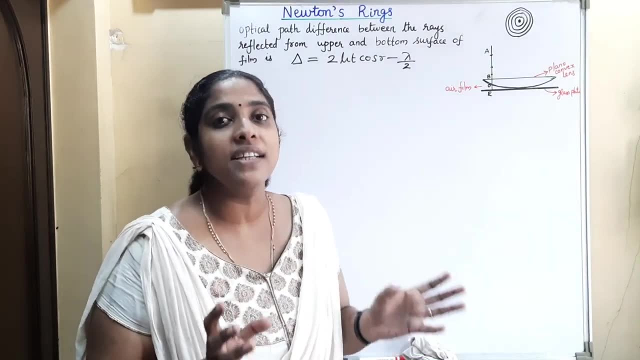 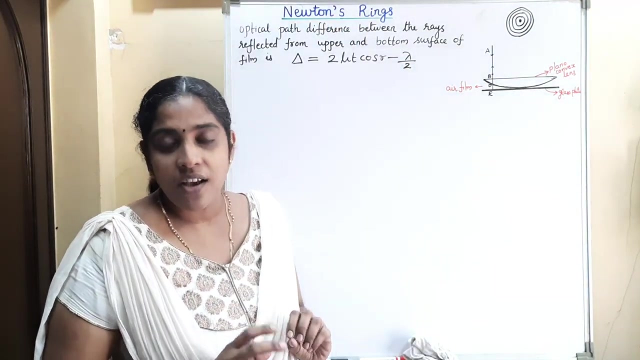 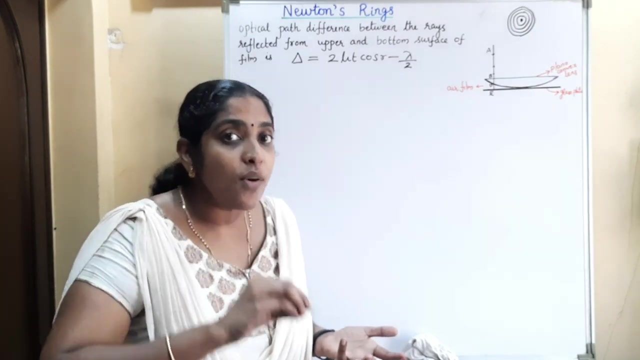 system we are observing through a travelling microscope, we can see a pattern like this. need bright and dark rings with a dark spot and the center. This pattern called Newton's ring. How these Newton's rings form, That is due to the interference produced because of the 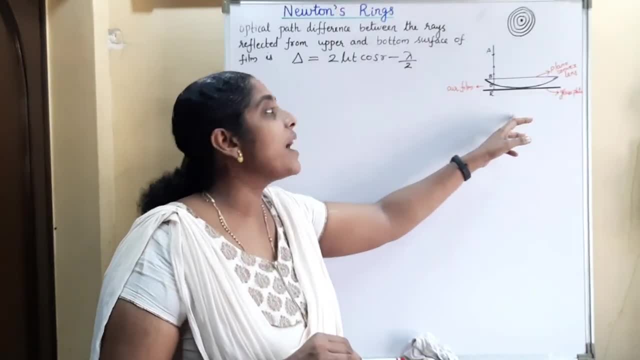 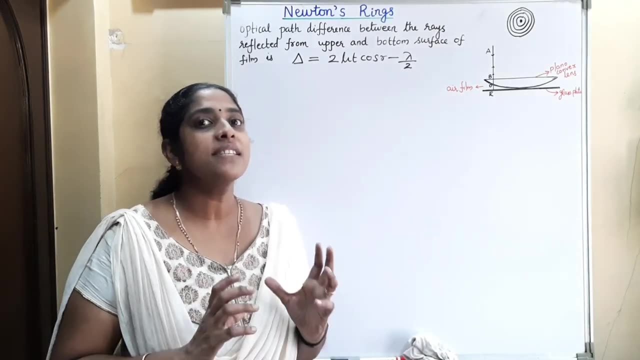 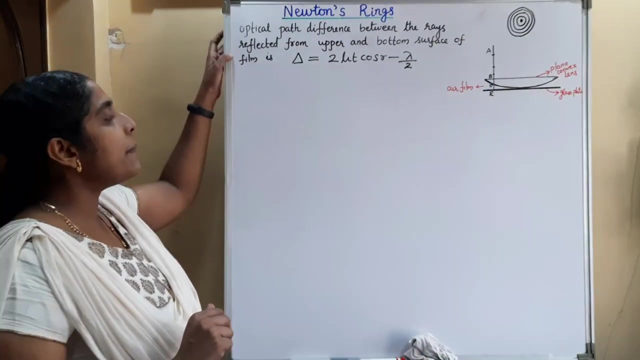 superposition of the light reflected from the top surface of the film and bottom surface of the film. To understand the theory behind it first, we can see the path difference between the light reflected from the upper and bottom surface of the film, So the optical path difference between. 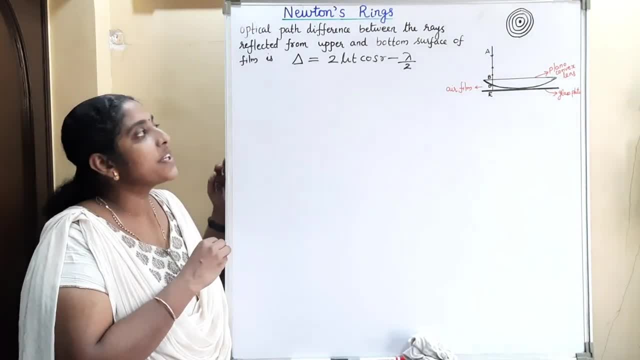 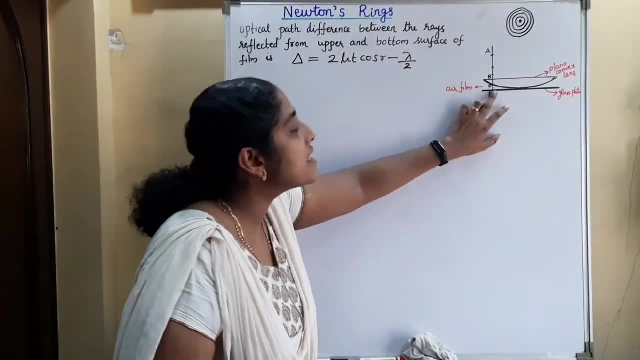 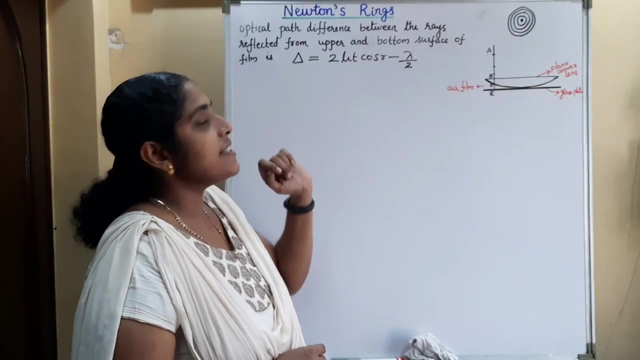 the rays reflected from upper and bottom surface of the film is: delta is equal to 2. mu t cos r minus lambda by 2, where t is the thickness of the film at what point we are considering, r is the angle of refraction and lambda is the wavelength of light used. mu is the refractive. 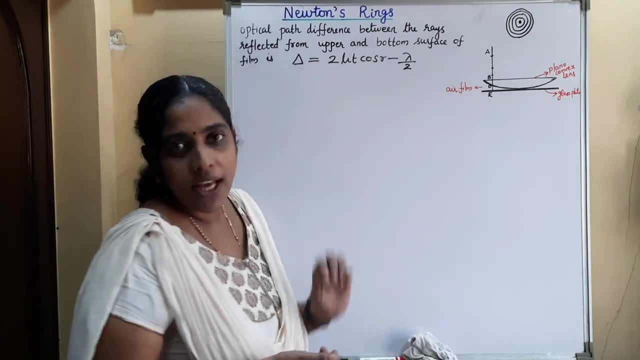 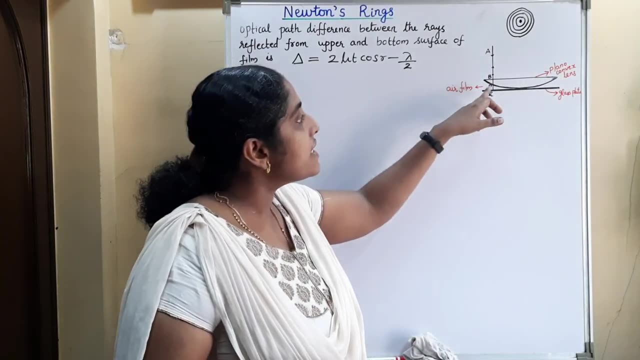 index of the film. So in this path difference we can see a lambda by 2 term. That lambda by 2 term arise due to the phase change. Where this phase change occurs. When the light get reflected from the upper surface of the film, the reflection occurs at 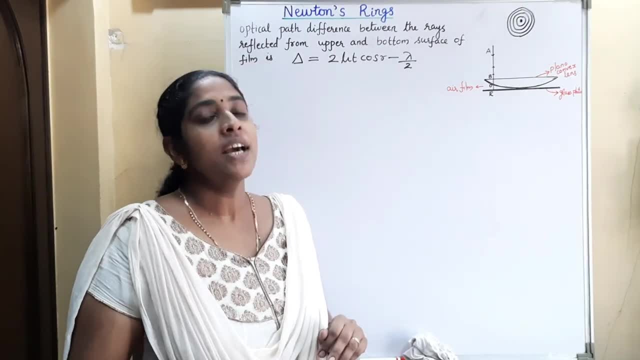 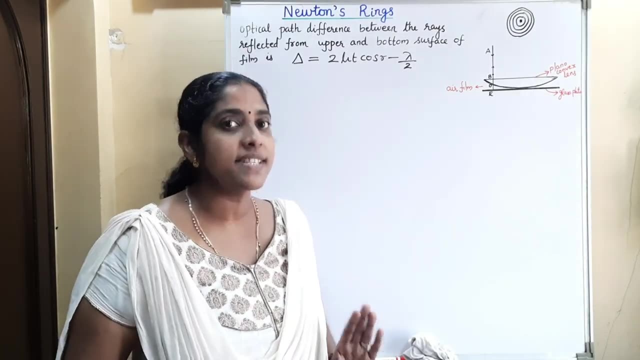 the glass to air boundary That is, denser to rarer boundary, When the light reflected from denser to rarer boundary. there will be no phase change. Therefore there will be no path difference correction there, But here, when the light reflected from the bottom surface of the film, 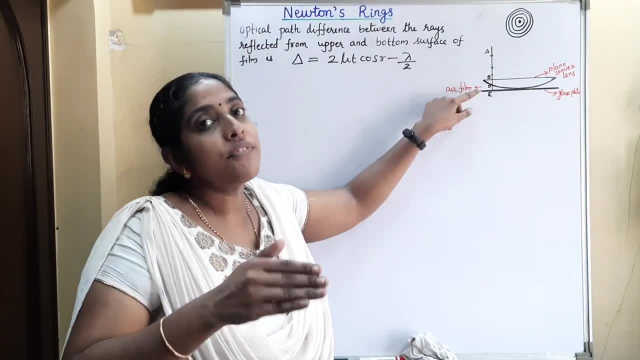 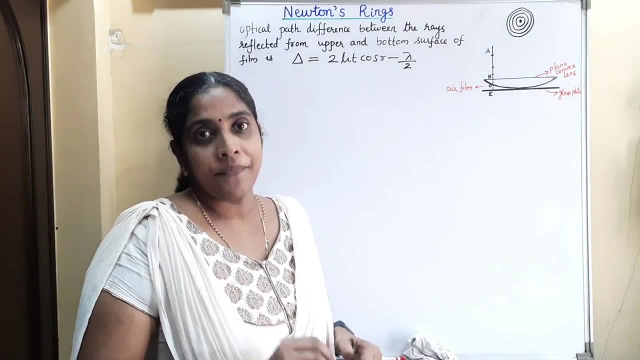 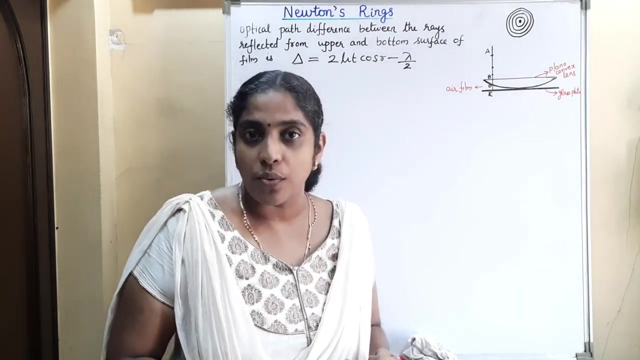 it is r to 2. glass boundary, that is, the reflection occurs at the rarer to denser boundary. that result into a phase change of pi. whenever the light reflected from the rarer to denser boundary, then there is a phase change of pi occurs. this phase change of pi is resulting into a path difference correction. 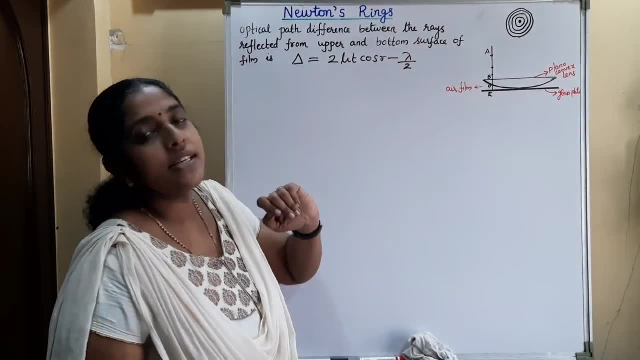 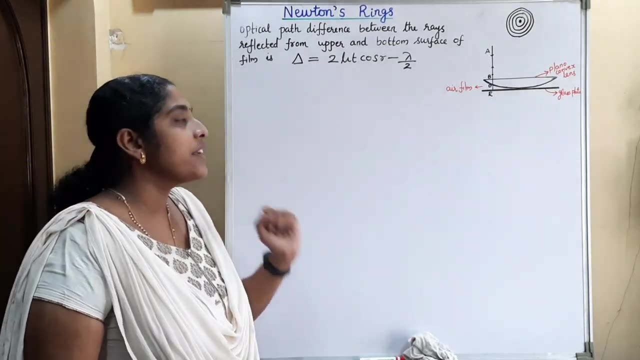 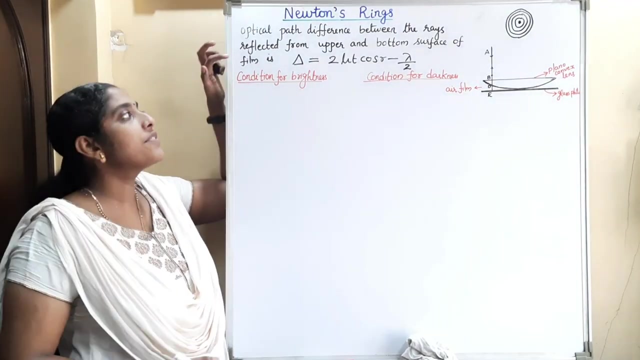 of lambda by 2, and here this lambda by 2 term is due to that phase change at for the reflected ray from the bottom surface of the film. so using this expression we can find out the condition for brightness and darkness in the newton string. so the condition for brightness is path difference. 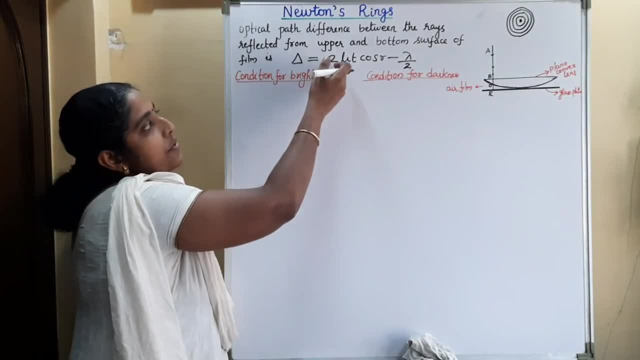 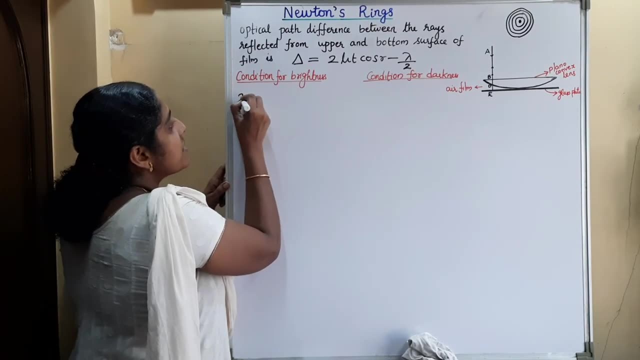 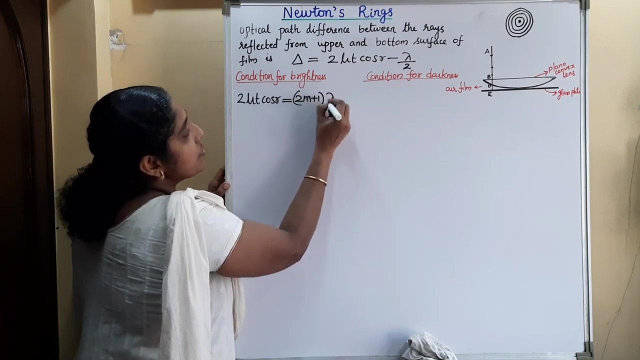 must be an integral multiple of wavelength lambda. so substituting this 2 mu t cos r minus lambda by 2 is equal to m lambda, and on rearranging we will get this condition as 2 mu t cos r is equal to 2 m plus 1 lambda by 2, and the condition 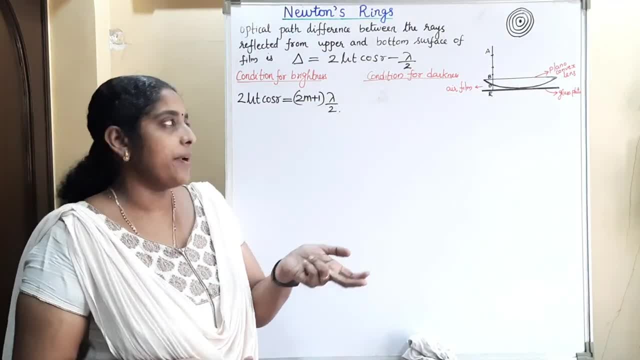 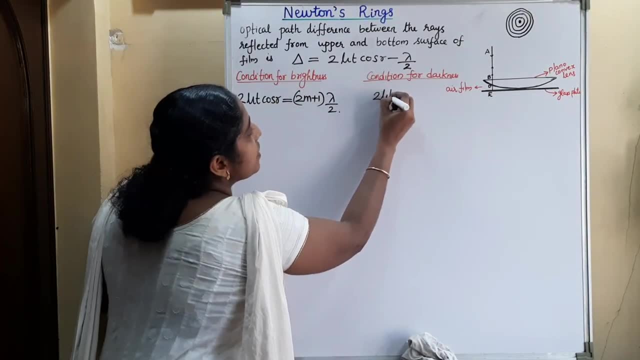 for brightness and darkness in the newton string is: path difference must be an integral multiple of lambda by 2. so on substituting this path difference into that expression, we will get this condition for darkness as 2 mu t cos r is equal to m lambda. now, if we are considering the 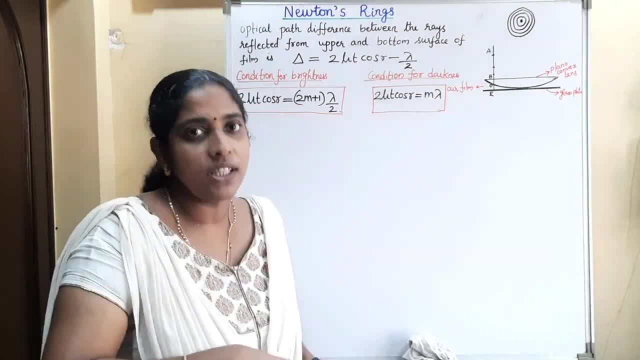 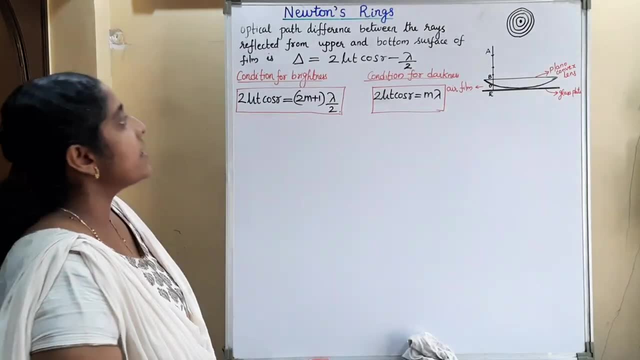 normal incidence of light. that is, if light is incident vertically normally, then the light will pass without any deviation. then the angle of refraction will be 0. that time we can consider this: cos r r r is equal to 2 mu t cos r is equal to 2 mu t cos r is equal to 2 mu t cos r is equal to. 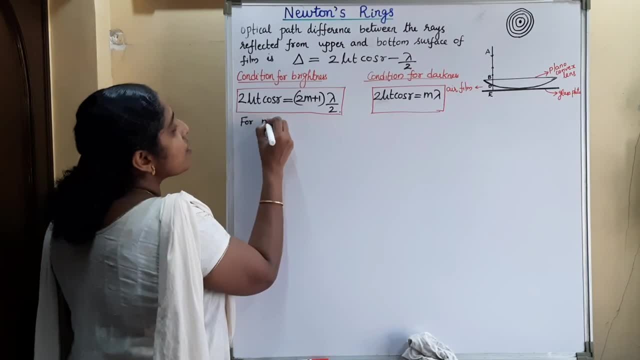 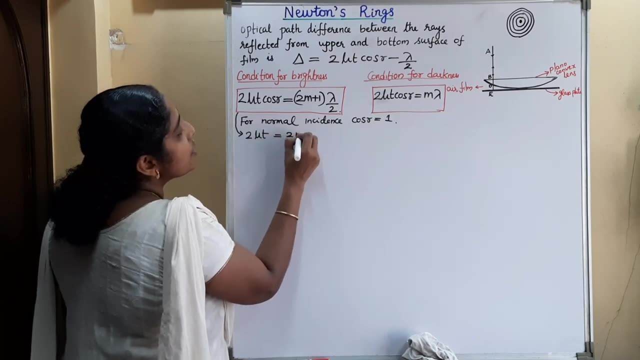 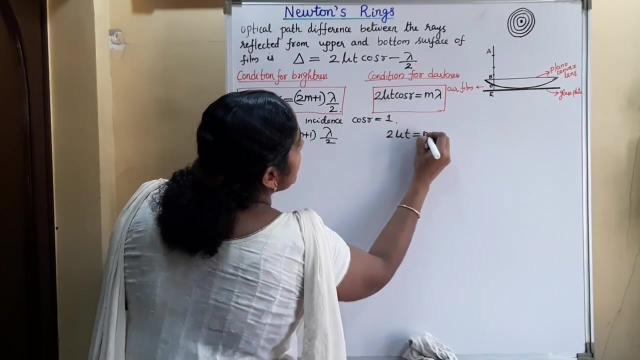 1. so for normal incidence, cos r equal to 1. so what will be this expression? so this expression becomes: 2 mu t is equal to 2 m plus 1 lambda by 2 for brightness, and 2 mu t is equal to m lambda. 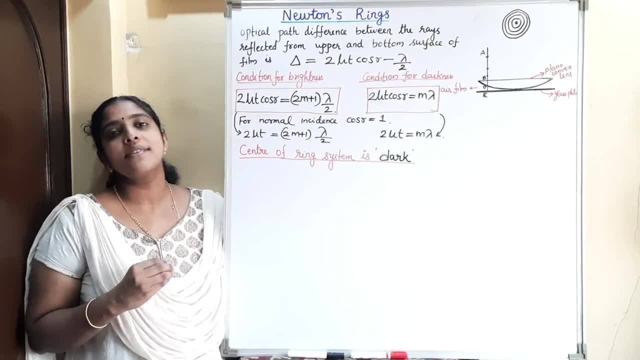 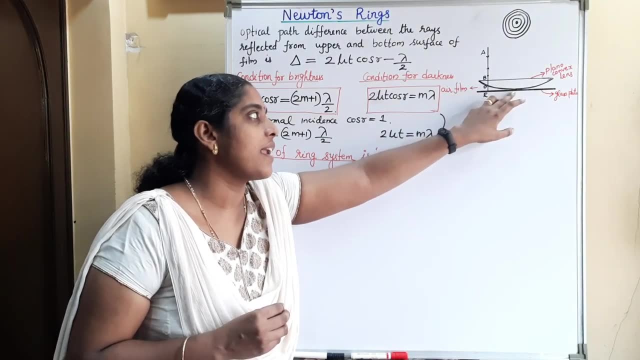 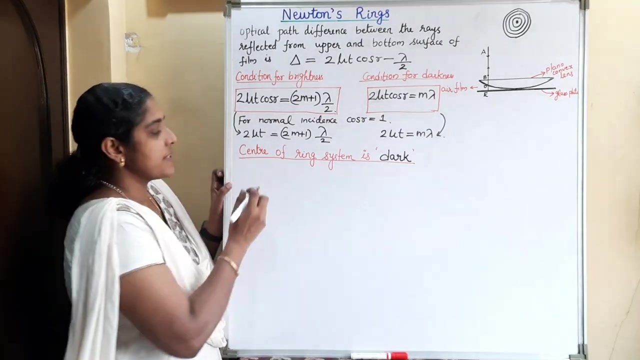 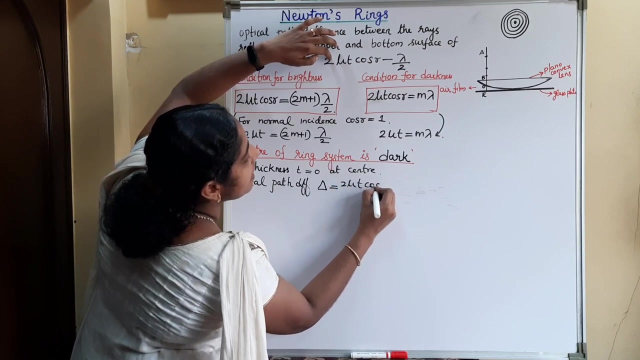 for darkness in newton string arrangement center of ring system is dark. why? because at the point of contact of lens and the glass plate thickness of air film is 0. if thickness is 0, what is the total path difference at the center? total path difference delta become 2 mu t cos r minus lambda 2 as minus lambda 2 because thickness is equal to. 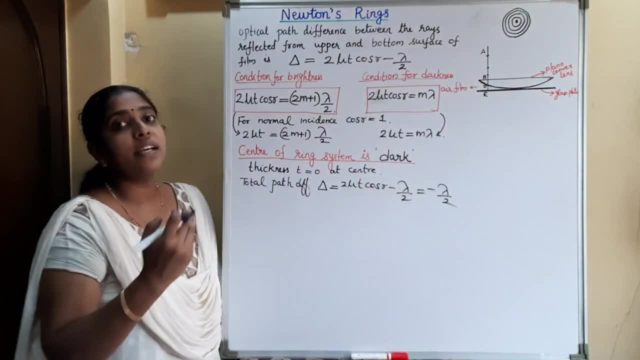 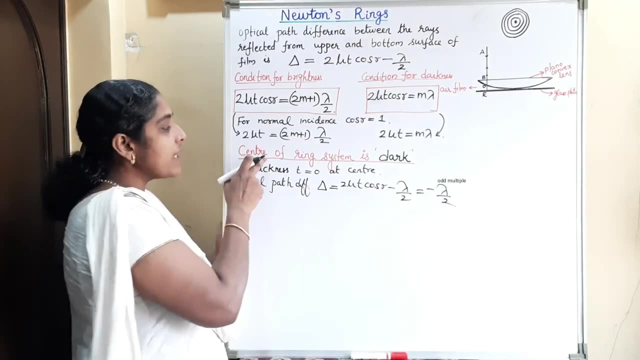 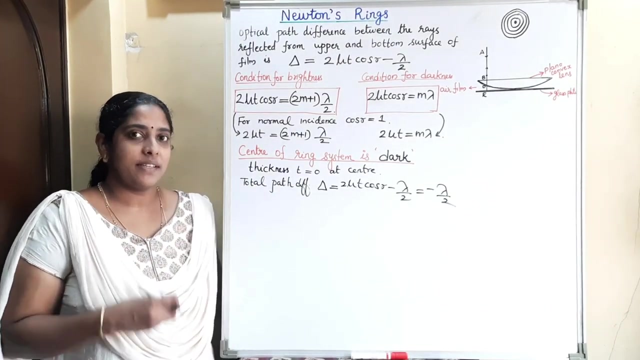 0. now the path difference is an integral multiple of lambda by 2. that corresponds to the condition of darkness. so at the center of the ring system we are getting dark spotter. if we study the transmitted system, that is, the interference producer due to the transmitted light, then also we will get a alternative: bright and 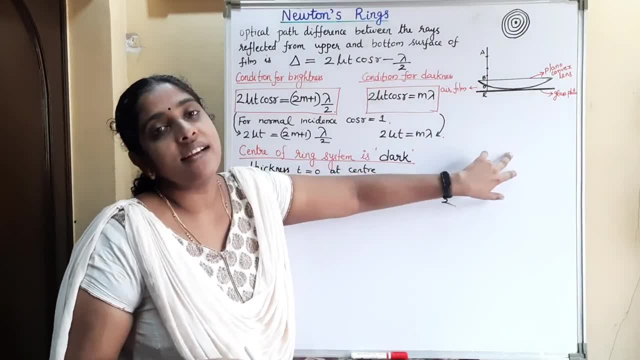 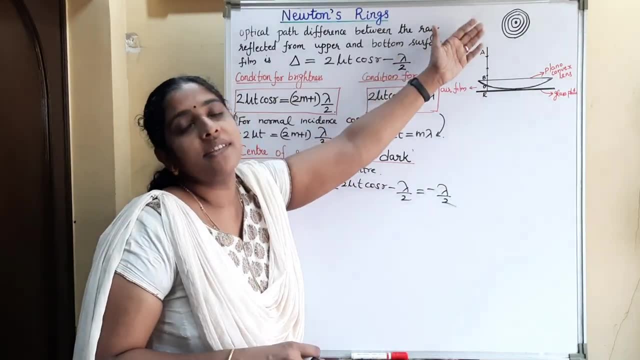 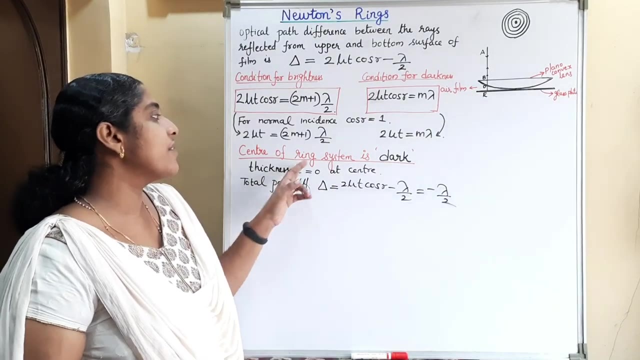 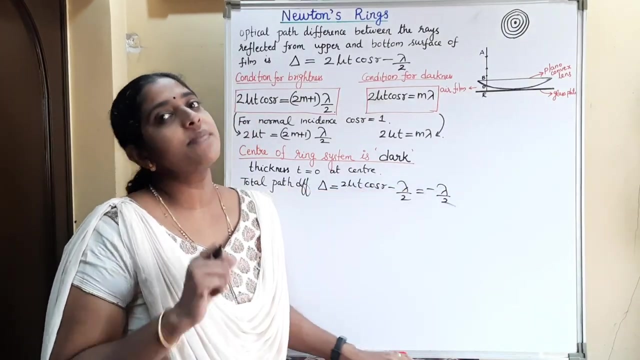 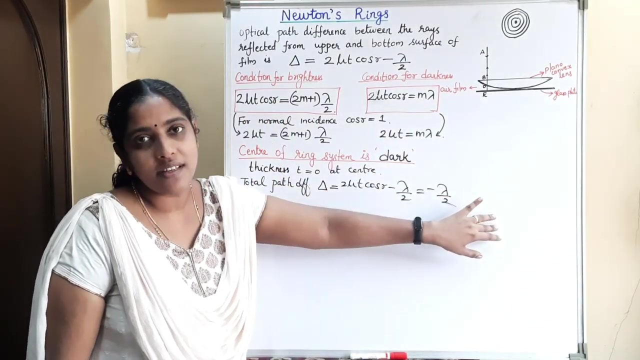 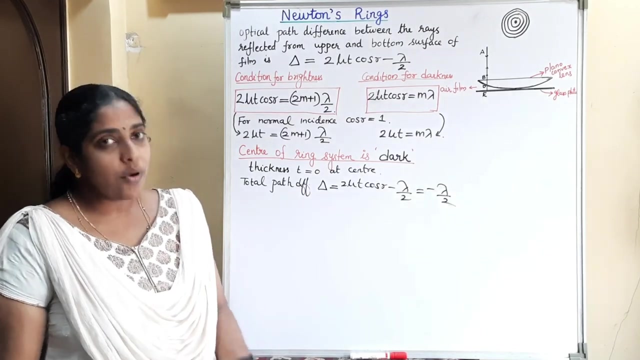 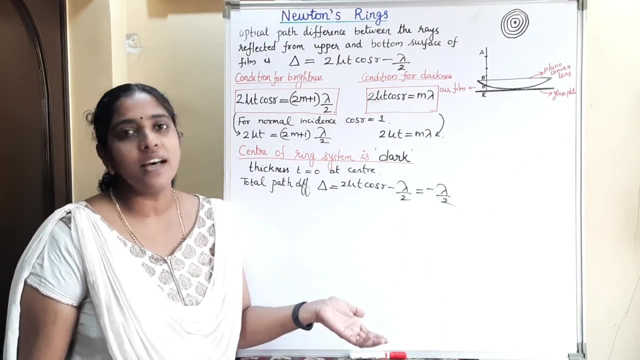 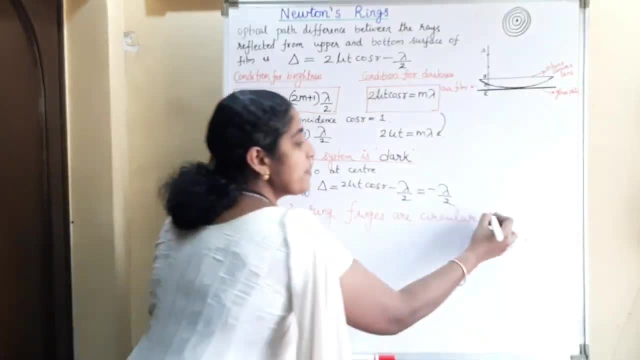 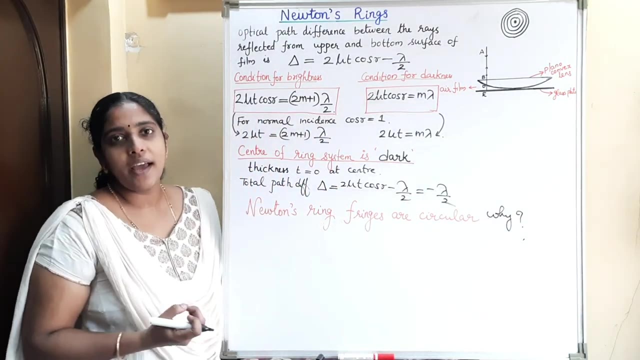 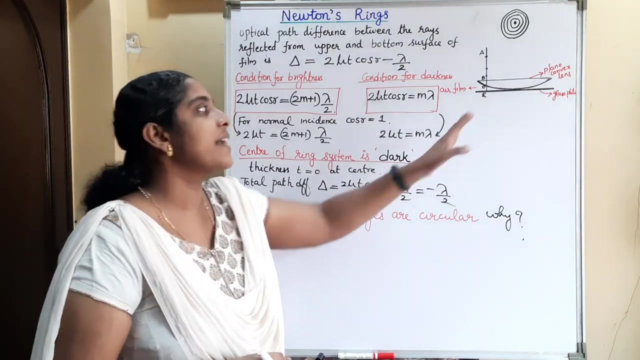 point is: newton's ring fringes are circular. why? from the name itself it is clear that in the interference pattern produced in newton's ring is circular. but why it happens? at the point of contact of the lens and the glass plate we are getting the dark spot. because the reason is that 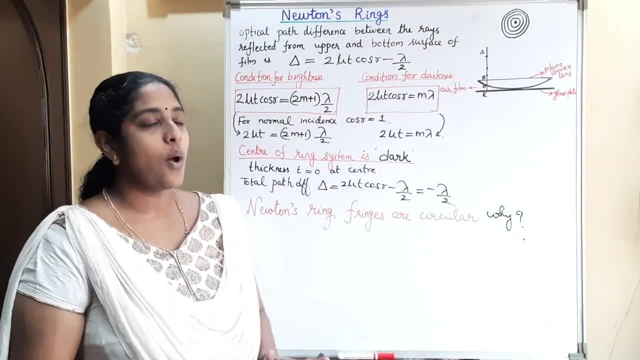 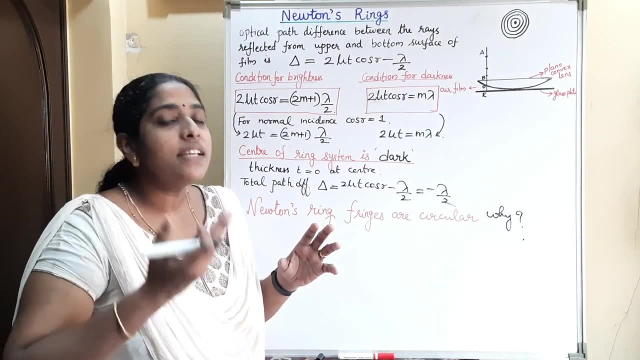 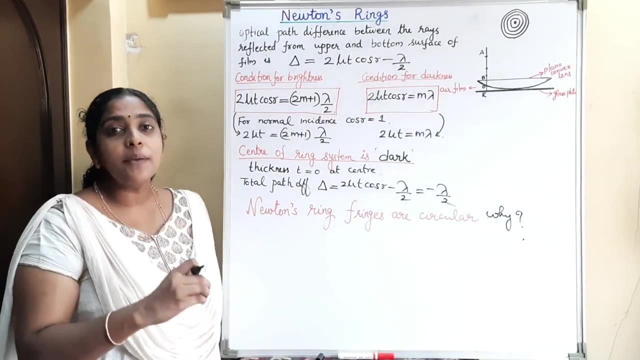 the thickness of the air film formed at the center is zero. but this thickness of the air film is progressively increasing outwards and this increase in the thickness is uniform all over the region. so if we take the points of same thickness around the center, we will get the 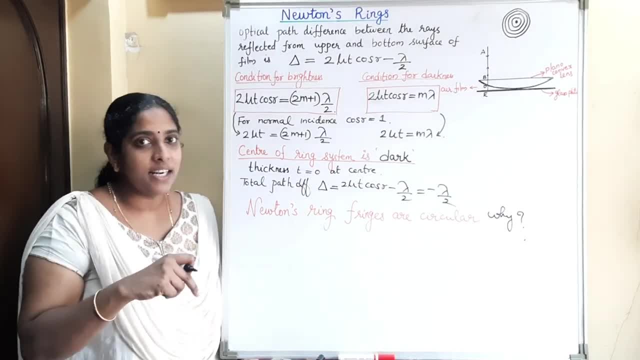 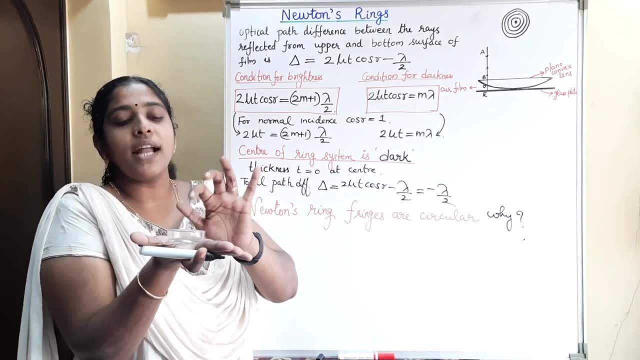 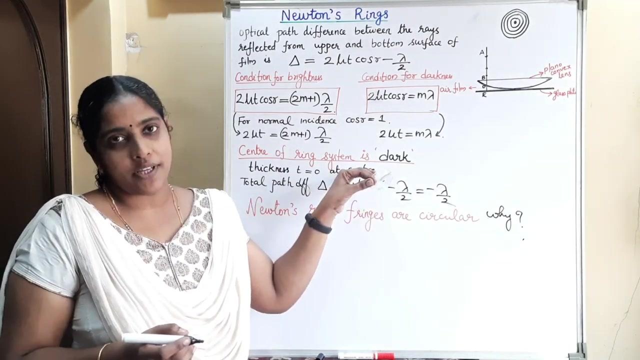 locus of all that points as a circle. let it be a planoconvex lens. so when this lens is placed over a plain glass plate, so at the center, the thickness of the air film formed is zero, so we are getting a dark spotter. but if we consider the points of same thickness outwards, then the 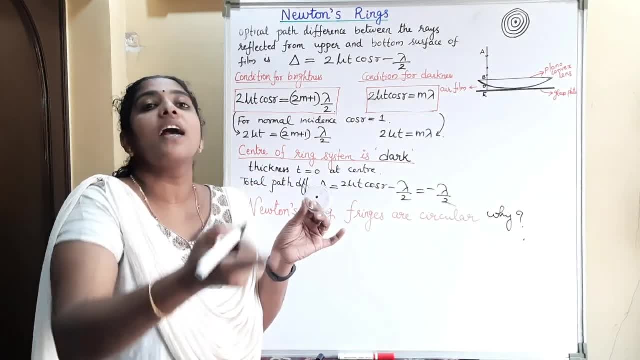 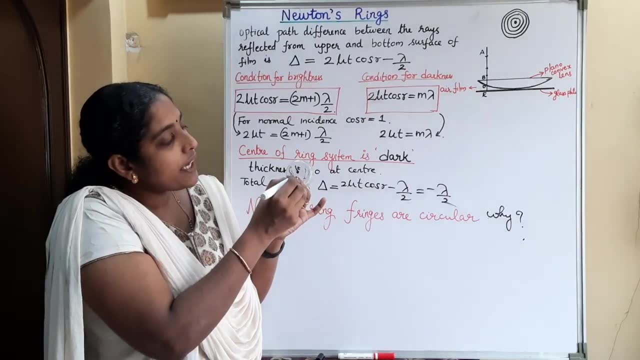 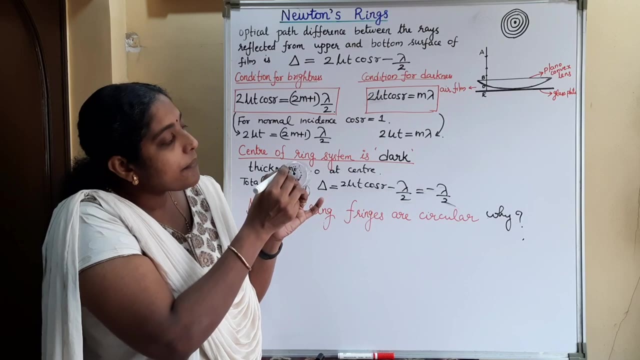 locus of all points have same thickness will come along a circle. that is, if i am taking a point here, this is having a thickness t. so if we take the points with the same thickness, the locus of all those points will come along a circle, with the center as the point of contact. therefore, the 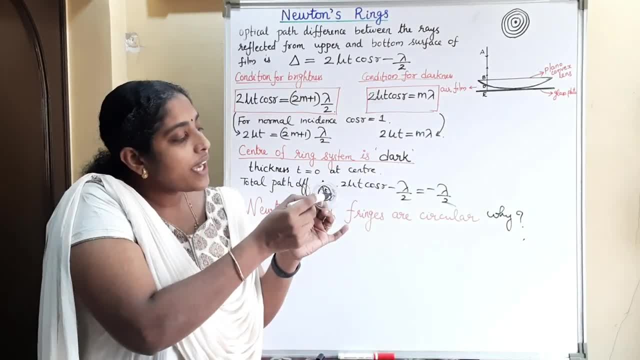 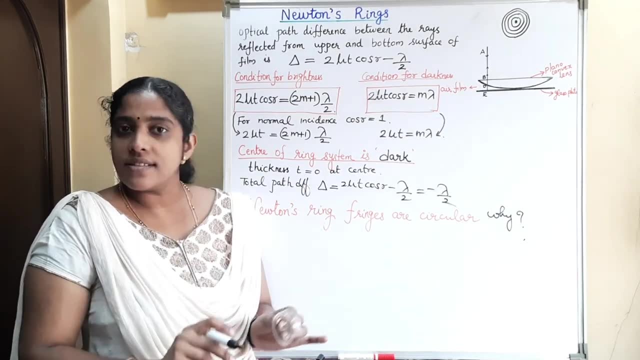 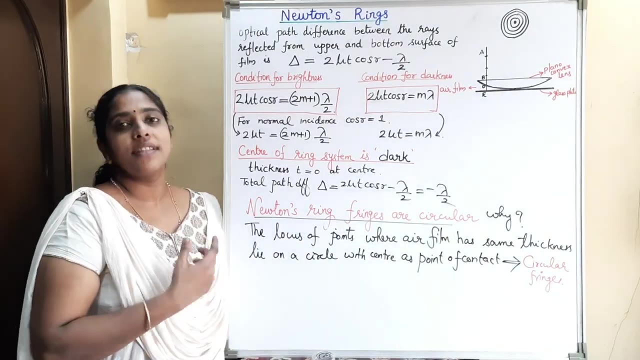 newton's ring fringes are circular. so if we are consider any circle in the newton's ring pattern, along that circle the thickness is constant. so the locus of points where air film has same thickness lie along a circle, with the center as the point of contact. therefore the circular fringes we are all getting a dark spotter. but if we take the points of same thickness outwards, then the locus of all points will come along a circle with the same thickness as the point of contact. therefore the newton's ring fringes are circular. so if we are considering any circle in the newton's ring, 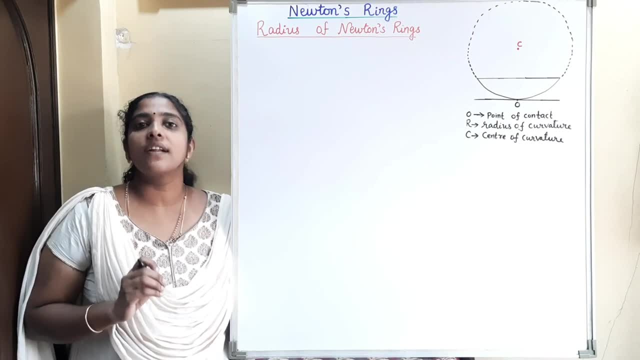 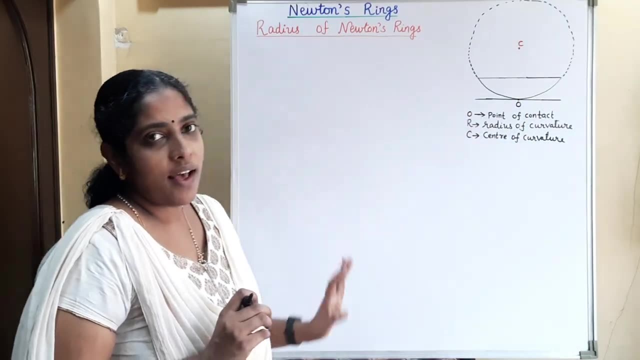 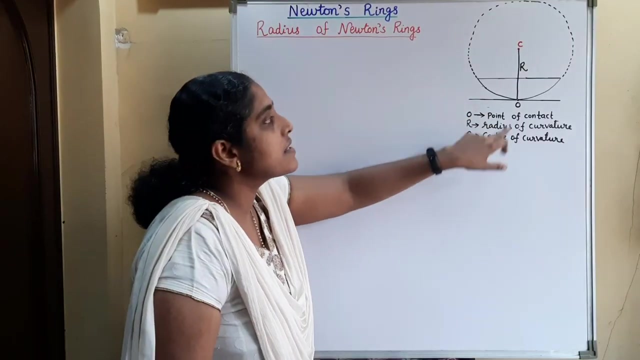 arrangement. now we can derive an expression for the radius of newton's ring. so here we have considered the plane of convex lens that is placed over the glass plate. this plane of convex lens is a part of a circle, so we are completing that circle by a dotted lines here. c is the center. 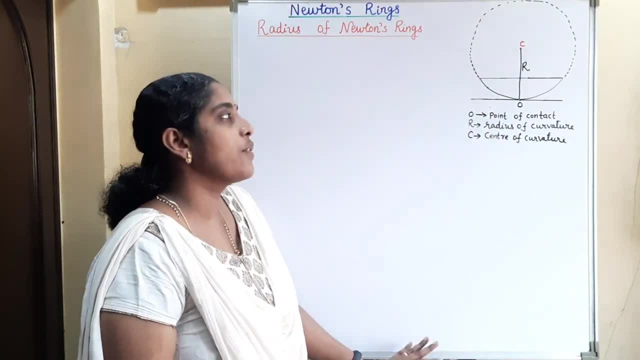 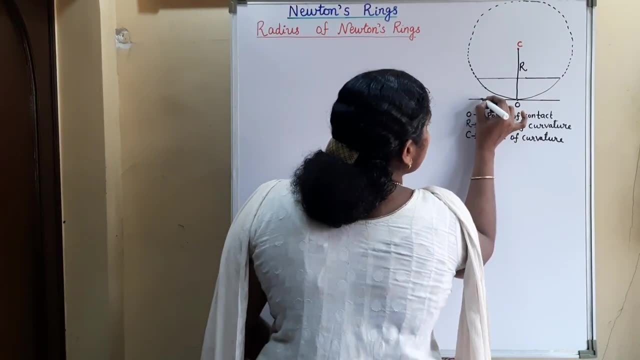 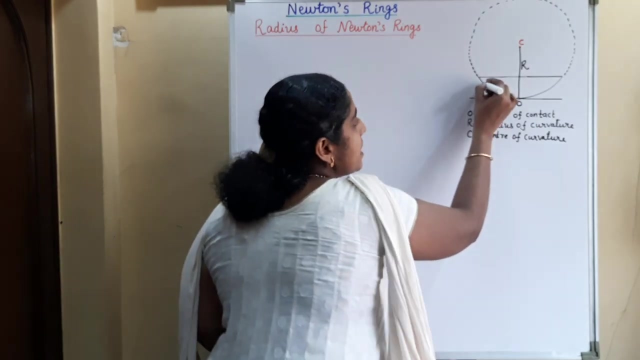 of curvature, and r is the radius of curvature of this plane of convex lens. now to find out the expression for radius of newton's ring, we can consider a point here. let at the point e mth dark band. of course, let t be the thickness of the air. 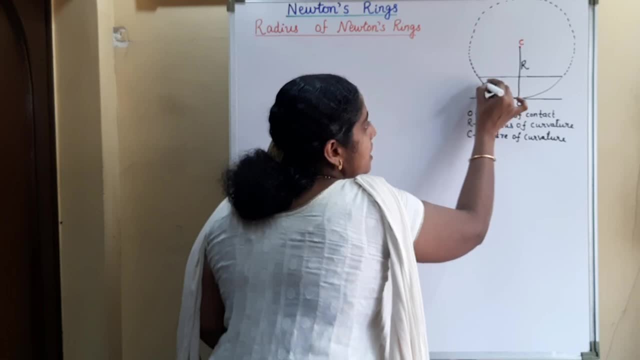 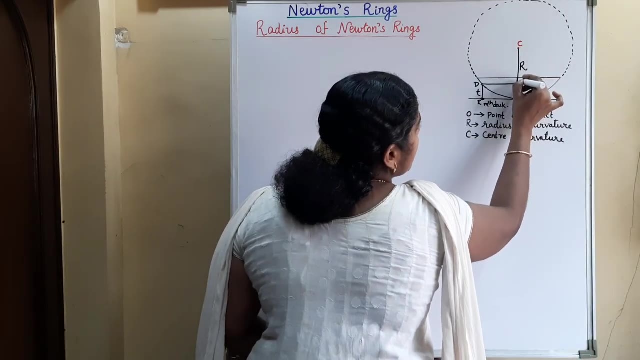 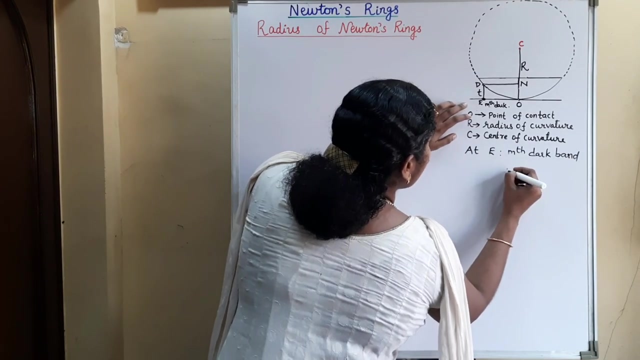 film formed at the point e. then let this point be d, we can draw a normal 2 o c. let it the point be n at e we are getting mth dark band. so the radius of that mth dark band is r e m. that means 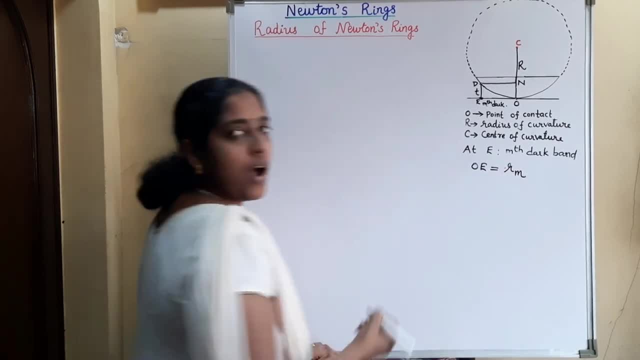 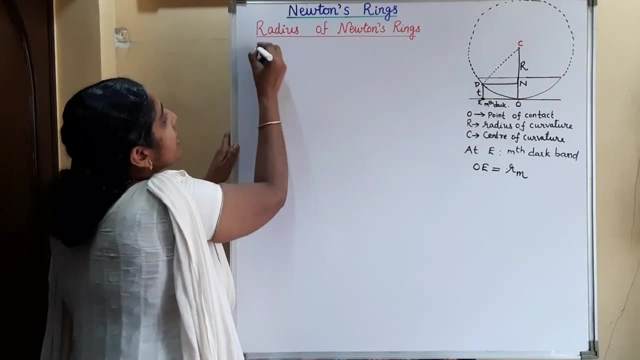 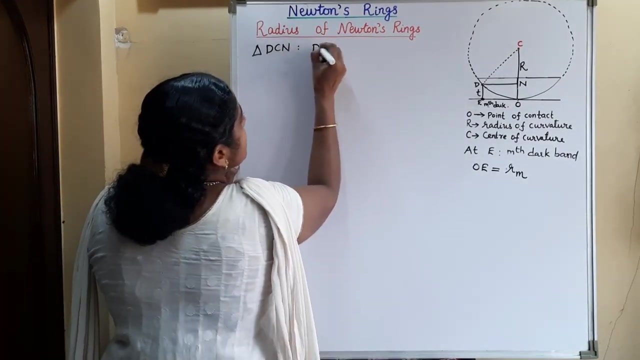 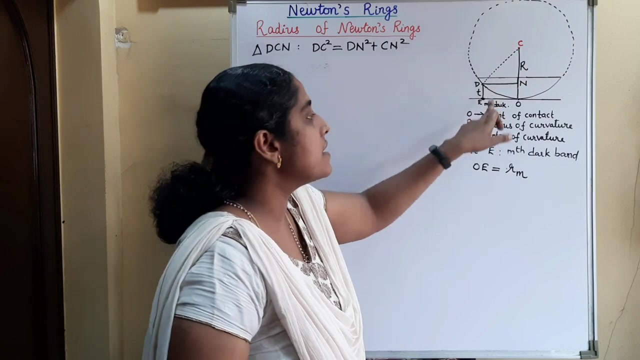 this o v distance is equal to r m. now we can consider a right angled triangle d c n. so in the right angle triangle d c n we can apply the pythagoras theorem, that is, d c square is equal to d n square plus c n square. what is this? d c, d? c is the radius of curvature of the lens, so d c square. 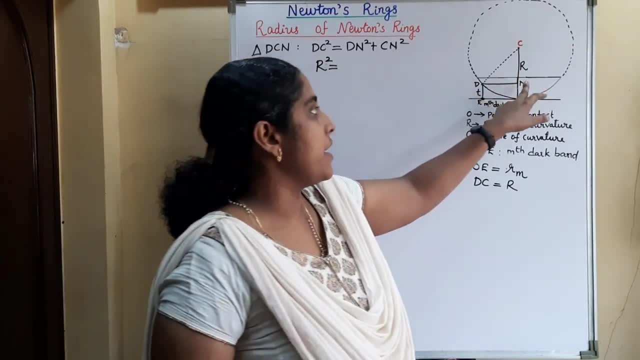 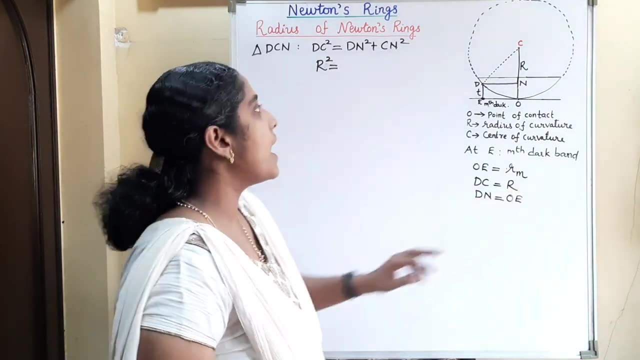 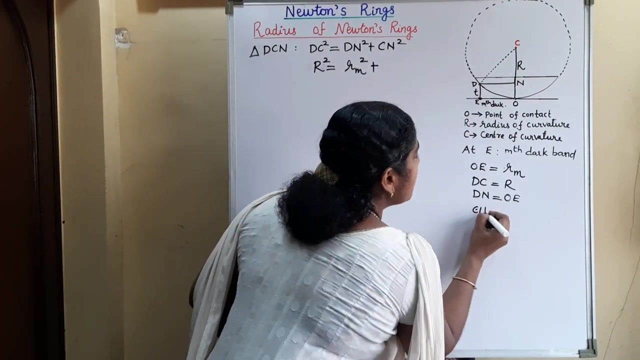 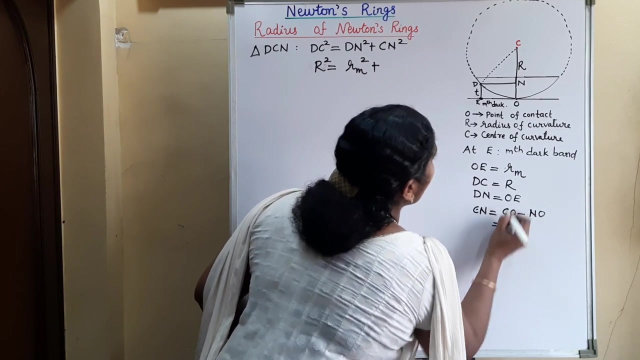 r square is equal to d? n. d? n is same as o? e, that is the radius of the mth dark ring there. so we can write d? n square as rm square plus c? n. so c n will be c? o minus n? o. what is this? c? o c? o is the radius of curvature, n? o is the thickness of the film at the point c? a. 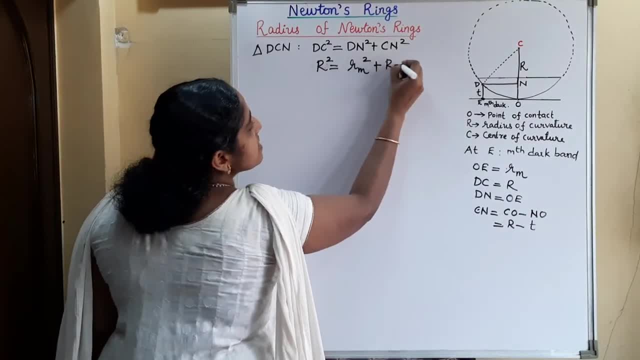 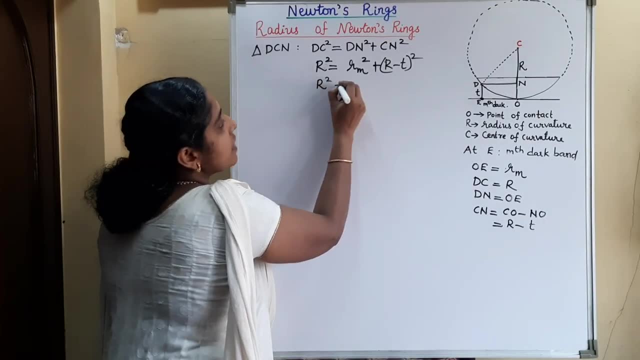 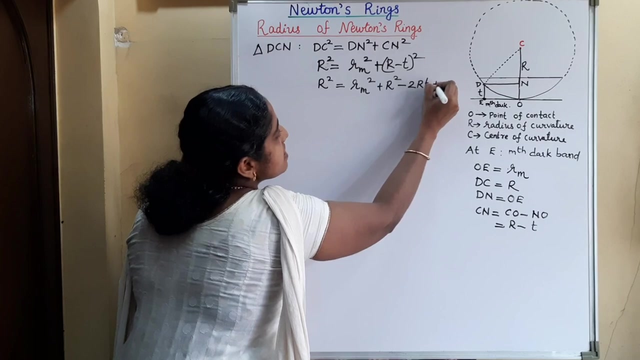 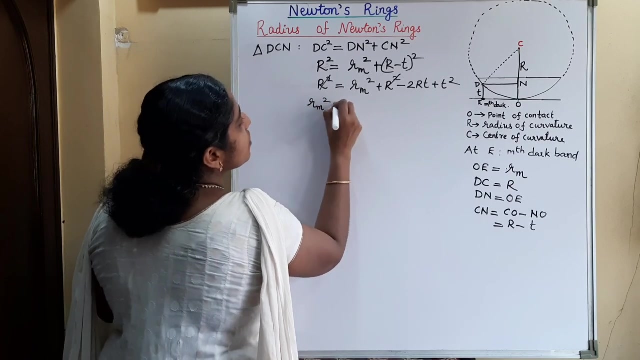 e. So cn is equal to r minus t. So cn square is r minus t, all square. Now we can expand this expression, that is, r square is equal to rm square plus r square minus 2rt plus t square. So this r square and r square will cancel and we will get rm square is equal to 2rt minus t square, Now this: 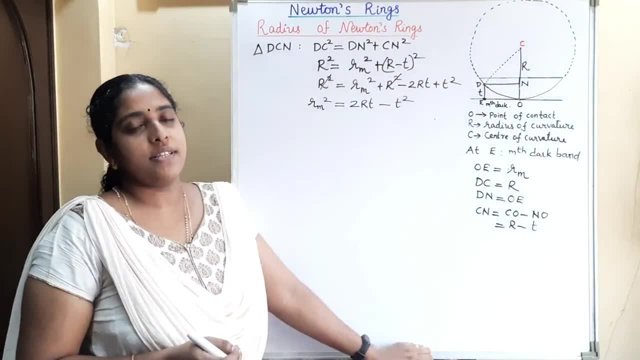 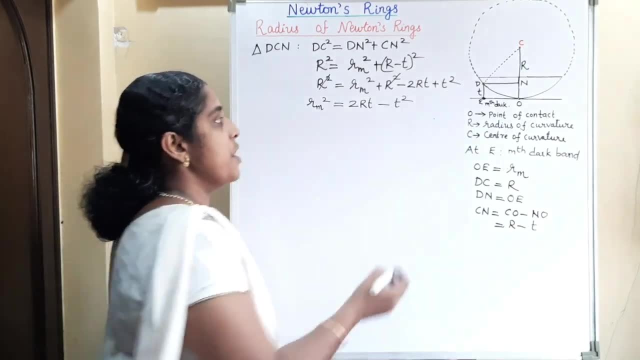 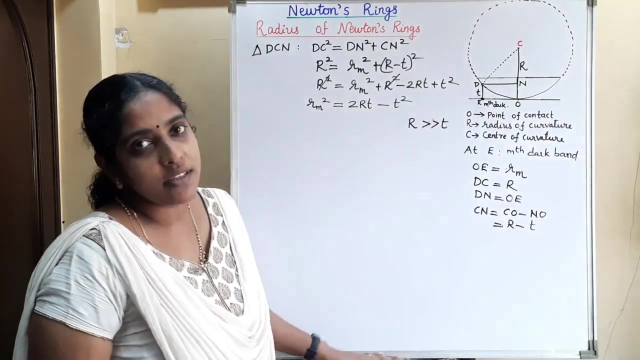 capital letter, r is the radius of curvature of this plano convex lens. In the Newton's ring arrangement we are using a plano convex lens of large radius of curvature. So if we compare this radius of curvature with the thickness of the air film, the radius of curvature is much larger than. 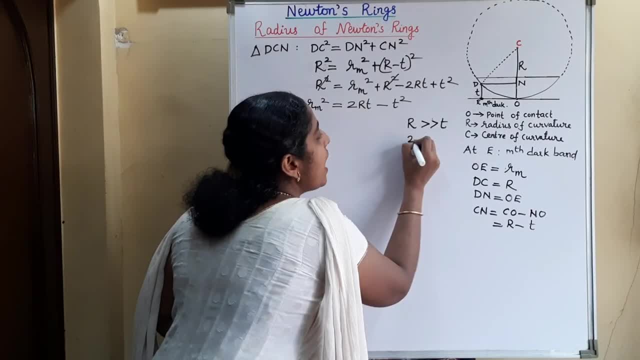 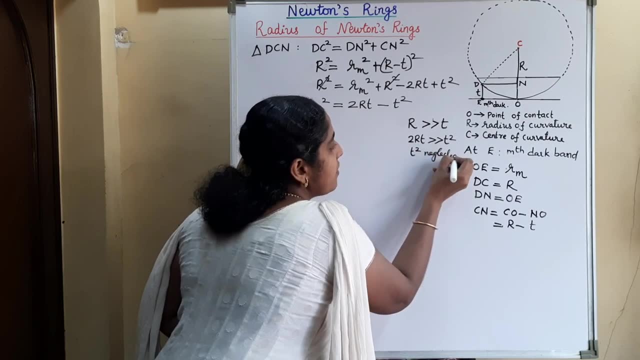 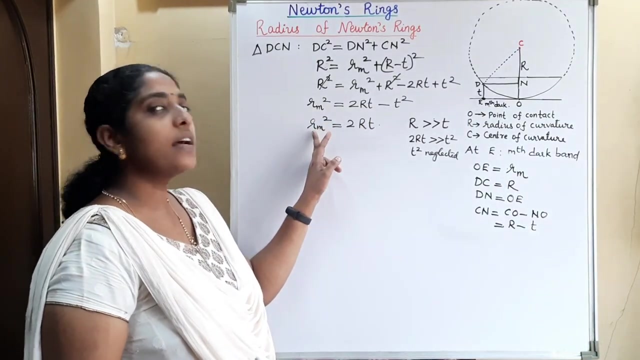 the thickness of the air film. So this 2rt will be much greater than t square and we can neglect the t square term here. So what will be this expression? rm square is equal to 2rt. Here rm is the radius of the mth dark ring. So the condition for 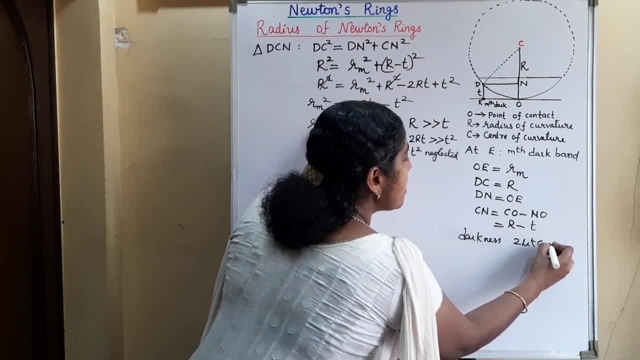 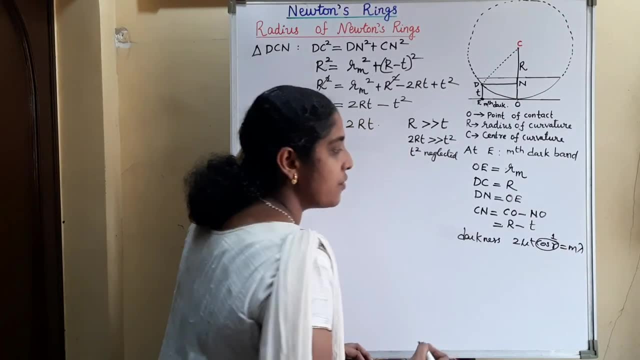 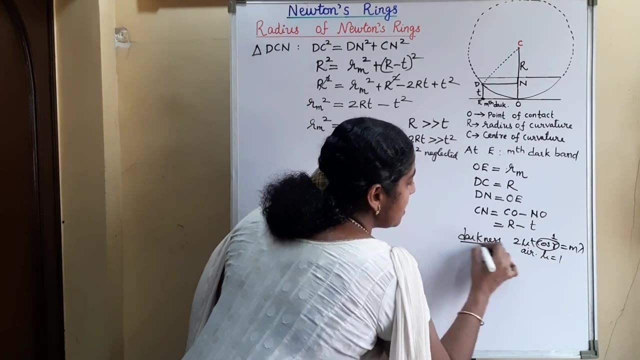 darkness is 2 mu t cos r is equal to m lambda. But in Newton's ring arrangement we are considering normal incidence. So this cos r equal to 1, and here the air for film formed is air, So air refractive index is equal to 1.. That is the darkness condition. here is 2t is equal to m. 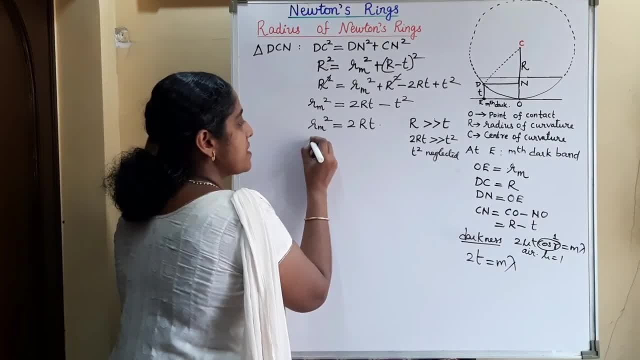 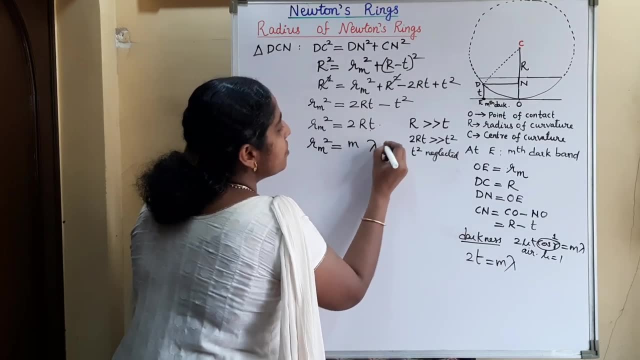 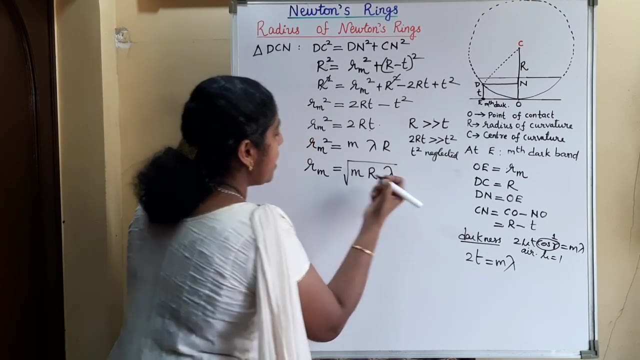 lambda. This 2t equal to m lambda we can substitute in this expression, that is rm square is equal to 2t, that is m lambda into r. Therefore radius of the mth dark ring is equal to root of m r lambda. So radius of mth dark ring in Newton's ring arrangement this rm is equal to root of m. 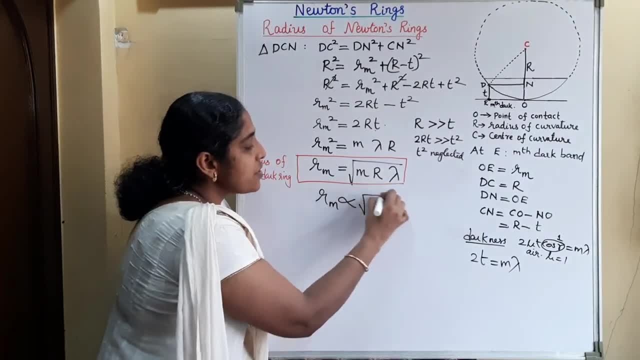 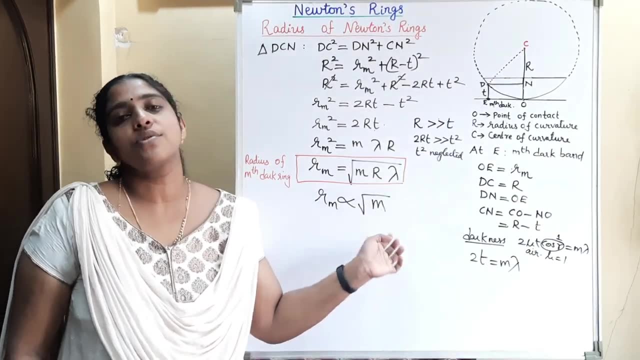 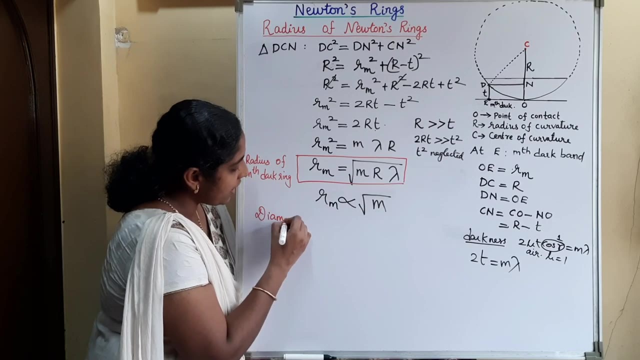 r lambda, That is rm is directly proportional to root m, That is, radius of rings In Newton's ring pattern is directly proportional to the square root of natural numbers. So from the expression of radius of mth dark ring we can find out the expression for diameter. 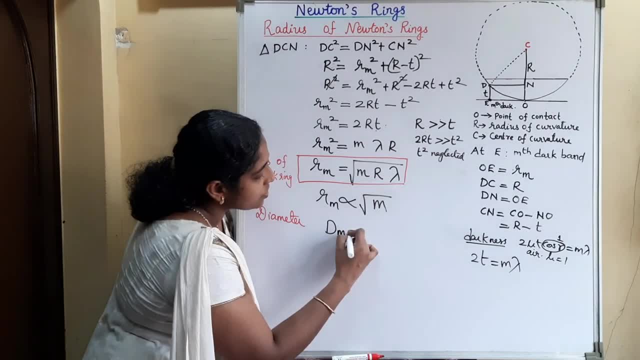 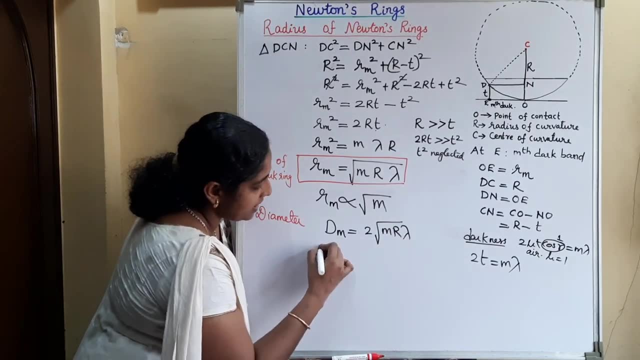 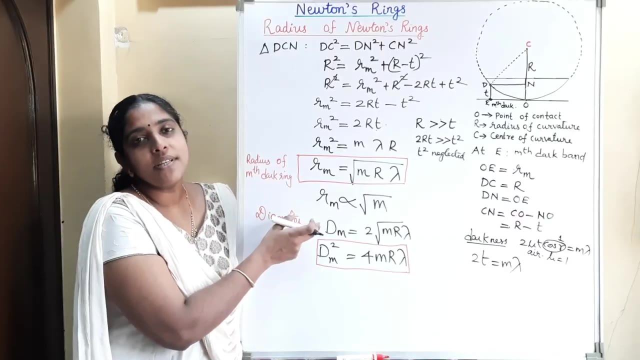 So diameter dm is equal to 2 times the radius. So 2 times root of m r lambda, or we can write it as: d square m is equal to 4 m r lambda. From this diameter expression we are getting an important point: that Newton's rings are not. 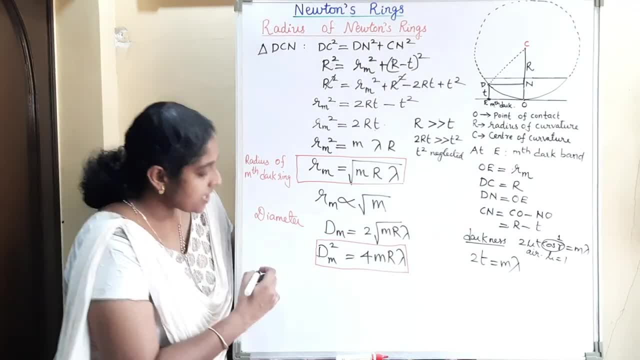 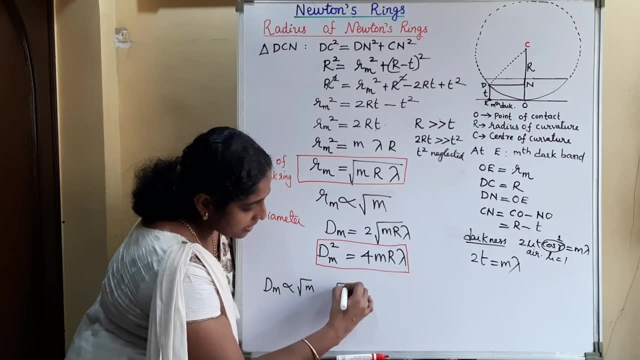 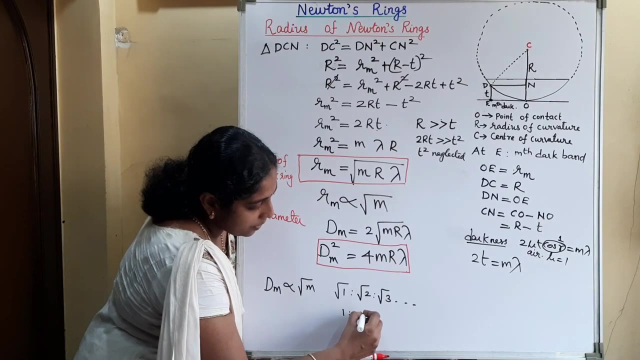 equally spaced. They are not even Means. if you are considering the diameter of ring, that is directly proportional to root m. That is, it is in the ratio. root 1 is to root 2 is to root 3, etc. That is here 1 is to 1.414 is to 1.732, etc. That means the space between two. 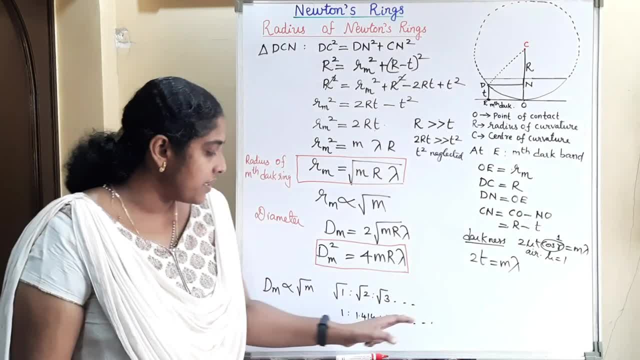 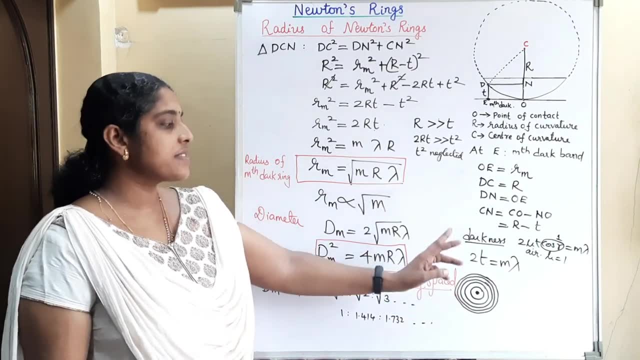 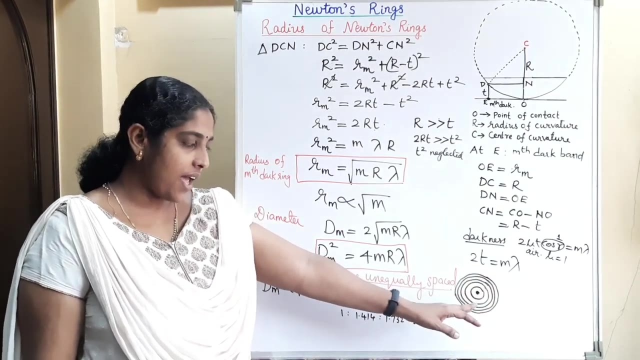 ring decreases as the order increases. Here the difference is .414. again that spacing decreases, That is, diameter of the ring pattern in Newton's arrangment does not increase in the same proportion as the order At the center. we are getting dark spotter after that. the spacing of the Newton ring is more near to the center. 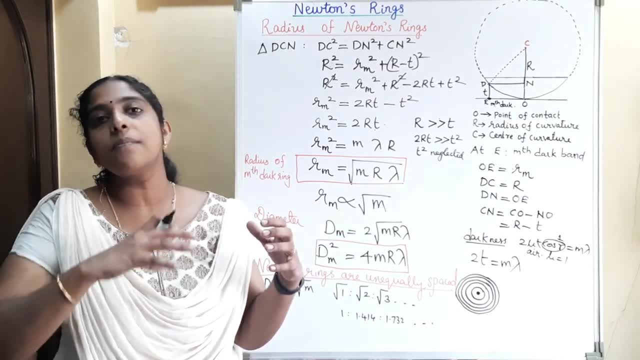 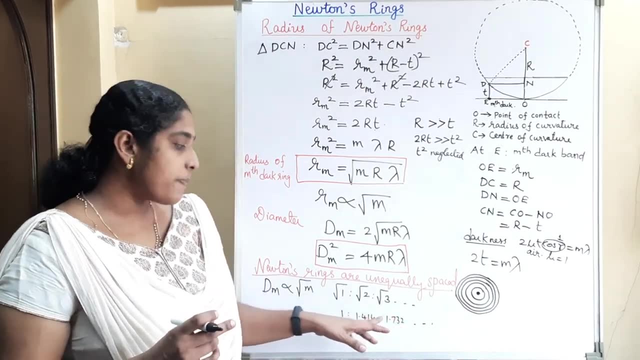 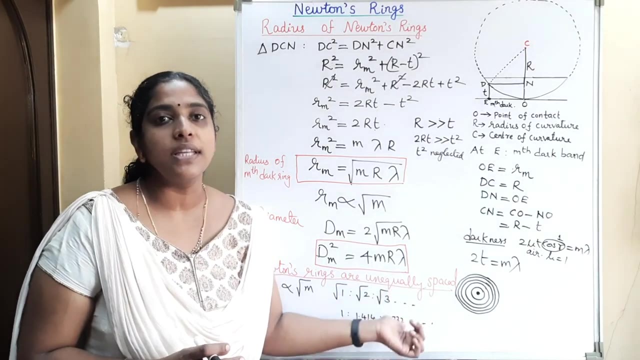 But that is as it is. more away from the center, Then this ring pattern become more and more close to each other, because as the order M increases, the spacing between the ring pattern decreases. so we can say that Newton's rings are unequally spaced. here we have considered: 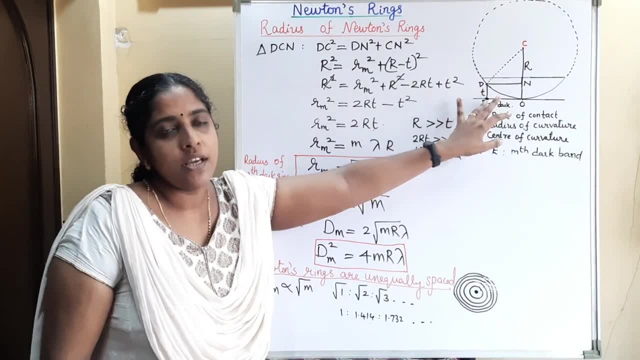 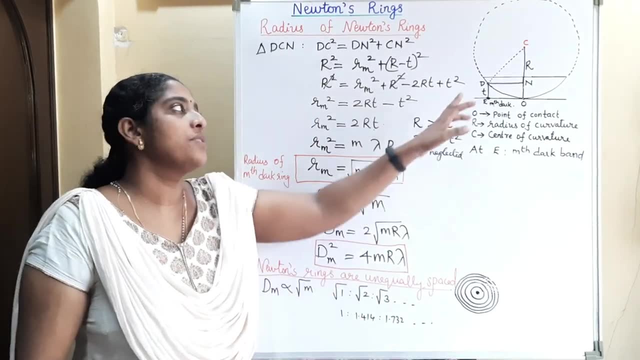 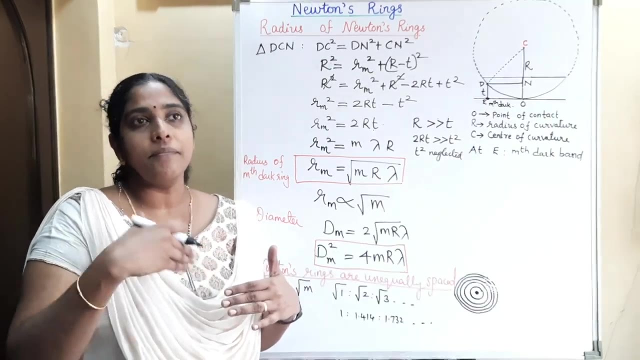 an air film between the convex lens and the glass plate. so if we keep a drop of liquid over the glass plate, a liquid film will form between the planar convex lens and this glass plate. then what will happen to the ring pattern? so if there is a medium in between this lens, 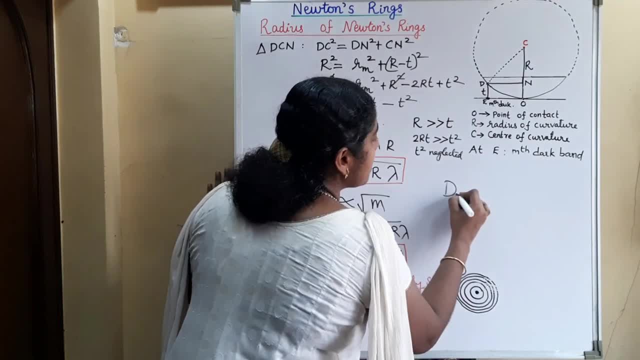 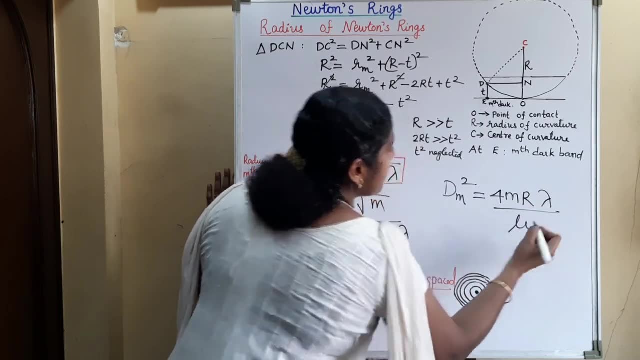 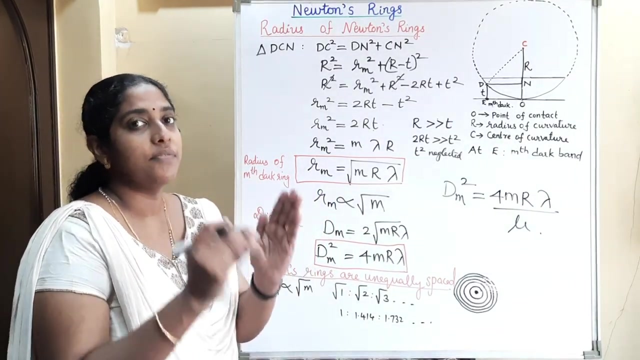 and this glass plate, the diameter of the ring pattern become 4mR lambda divided by mu, where mu is the refractive index of that medium. so what happens to the diameter of the ring pattern? if liquid is introduced between this glass plate and lens, then the diameter will. 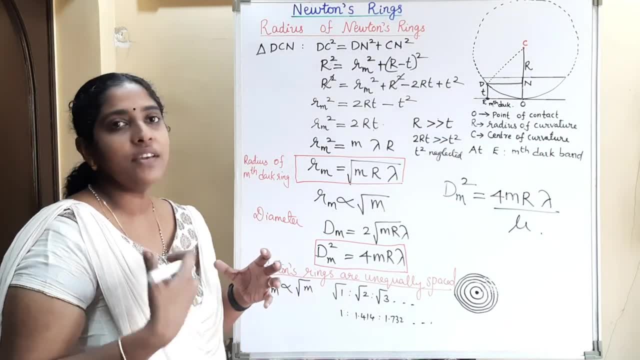 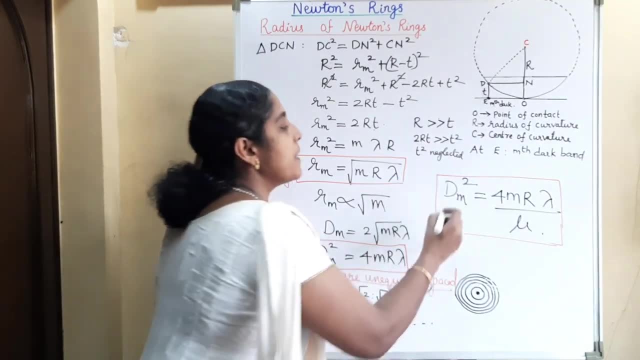 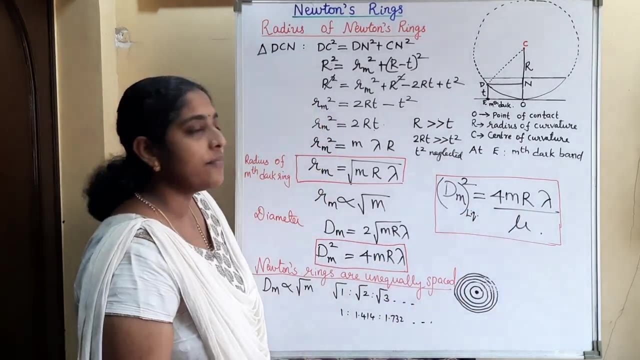 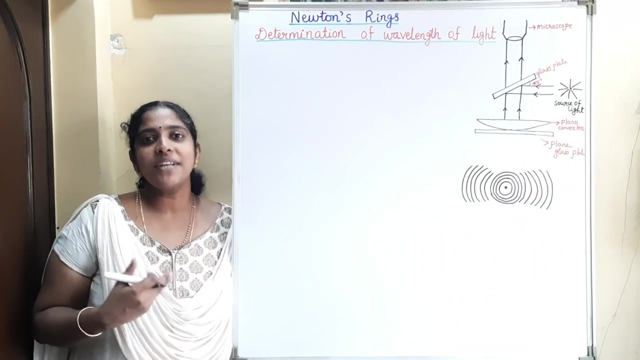 shrink, So that shrinking will depends upon the refractive index of the medium, so the diameter of the ring. if a liquid is placed between this glass plate and the lens, then the expression is d square M liquid is equal to 4mR lambda divided by refractive index of the liquid, one of the 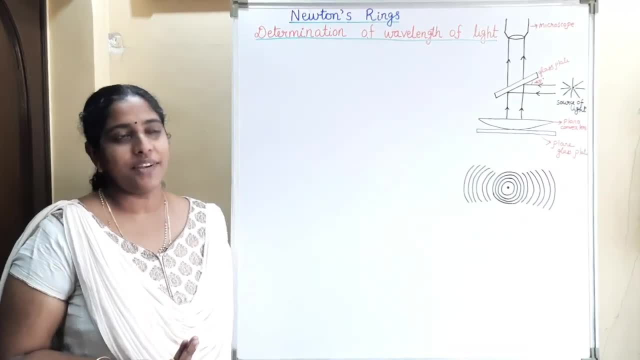 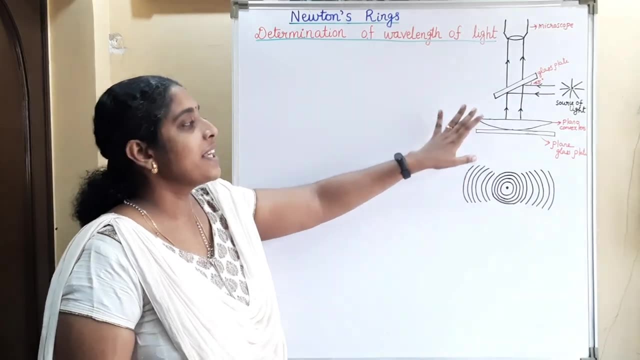 application of Newton's ring is determination of wavelength of light. we can see the arrangement of light at a 45 degree. so in my choice of the light we can take a plane or convex lens and a glass plate and keep the lens over the display of the glass plate. this system is 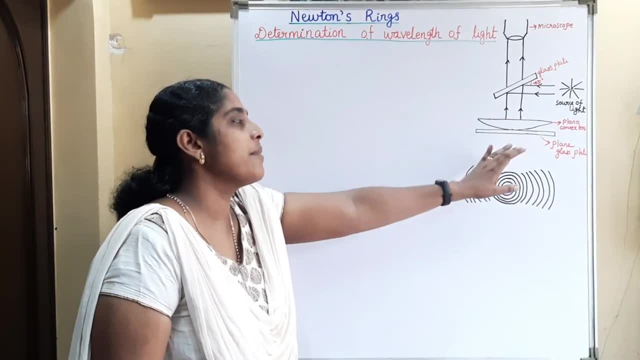 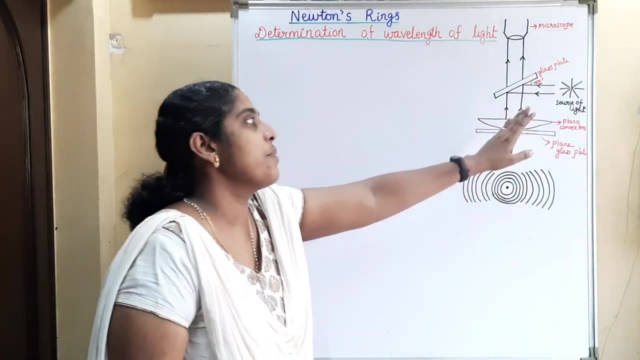 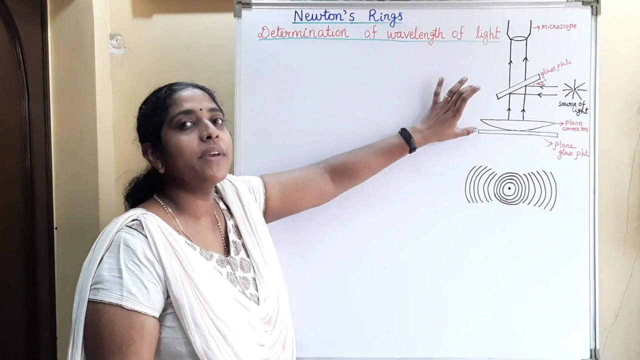 held under a travelling microscope and is placed before a monochromatic source of light whose wavelength we are going to determine, let it be sodium vapor number. when the light from the sodium vapor number is incident on a glass plate, here the glass plate is inclined at a 45 degree in order to make the normal incidence of light. so, when the light from 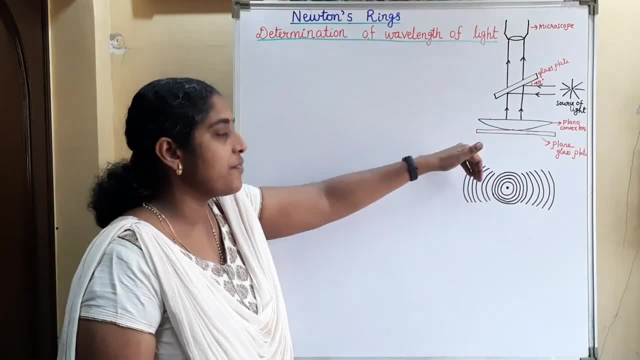 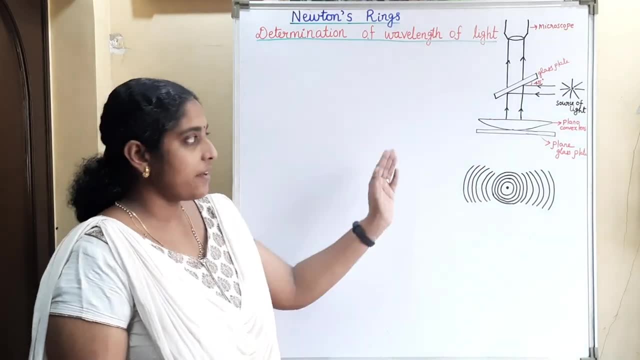 the source is incident on the glass plate. the light is kept on the glass plate and the on this glass plate it will get fold into the system and the light will get reflected from the upper and bottom surface of the air film between the lens and the glass plate. so the superposition. 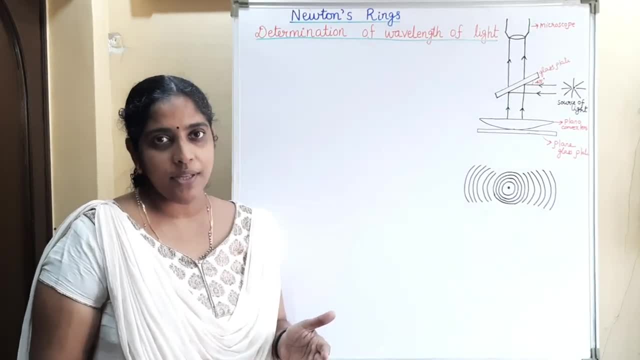 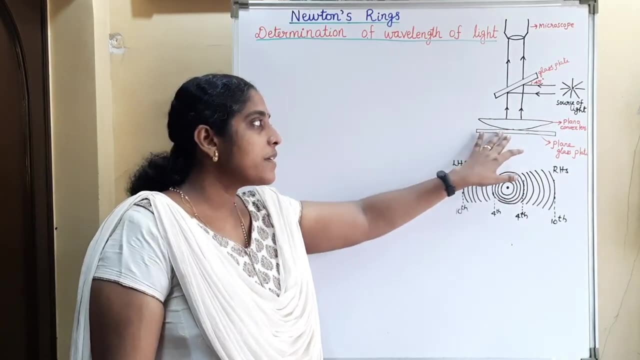 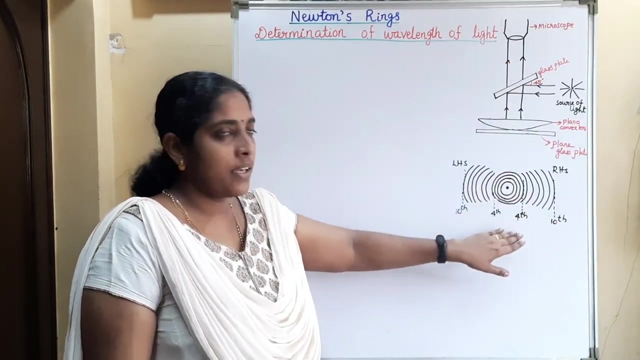 of the light reflected from the top and bottom surface of the film will produce an interference pattern and this interference pattern we can observe through this traveling microscope. while observing the interference pattern produced in this setup using the traveling microscope, we are seeing a ring pattern like this, so we can measure the position of various dark ring on the 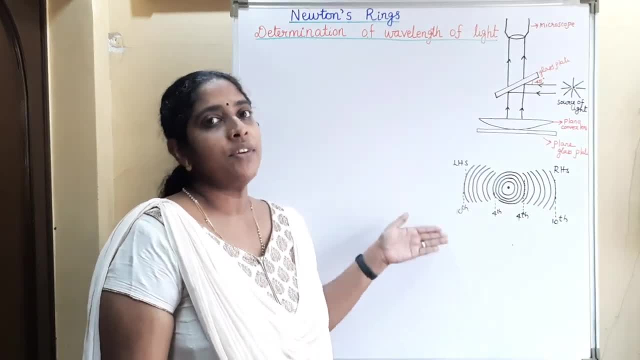 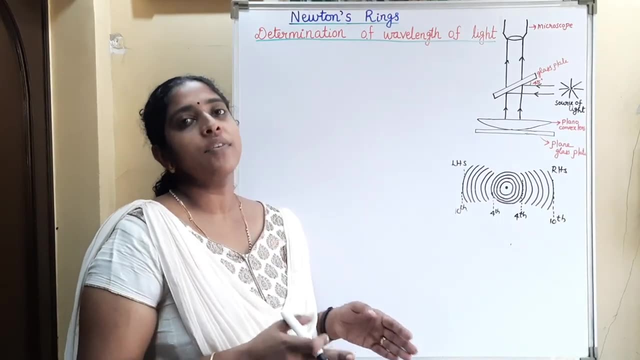 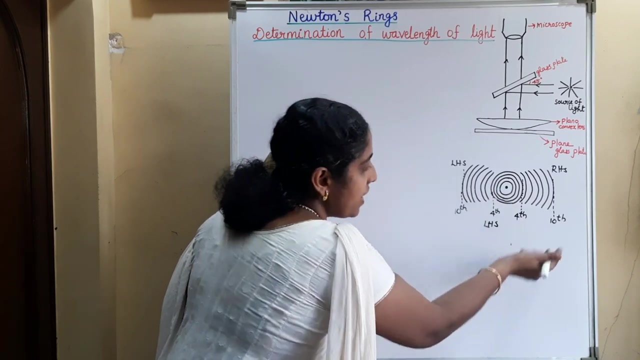 lhs and the rhs with the help of main scale and vernier scale in the traveling microscope in order to find out the position we are keeping the vertical crossbar in tangential with these ring pattern. so on, the lhs take the position of the fourth ring and also take the position of 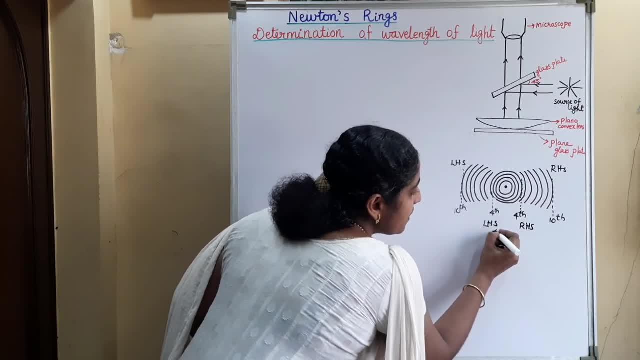 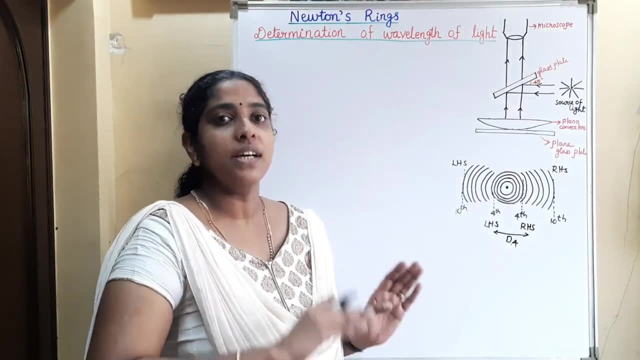 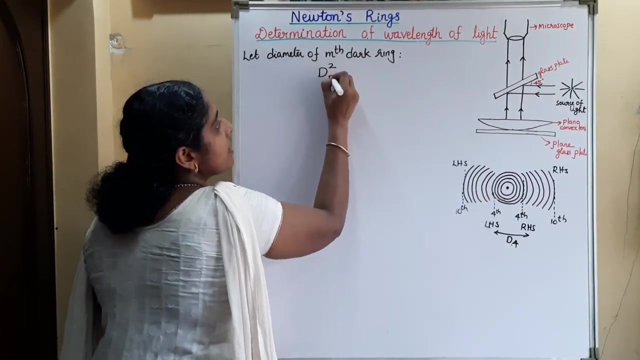 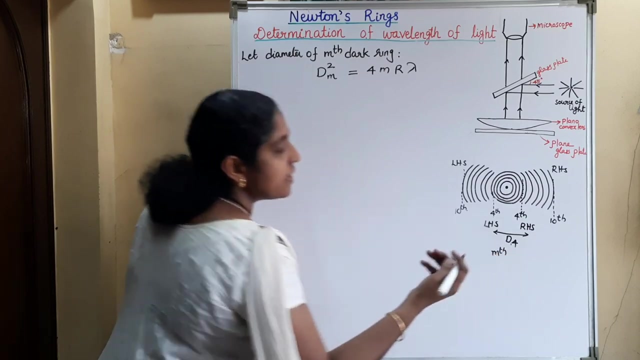 fourth ring on the rhs, then the difference between these two position will give the diameter of the fourth ring. similarly, we can find out the diameter of any ring in this interference pattern. let diameter of the mth dark ring is d square m is equal to 4 m r lambda. let this fourth ring be the mth dark ring and we can. 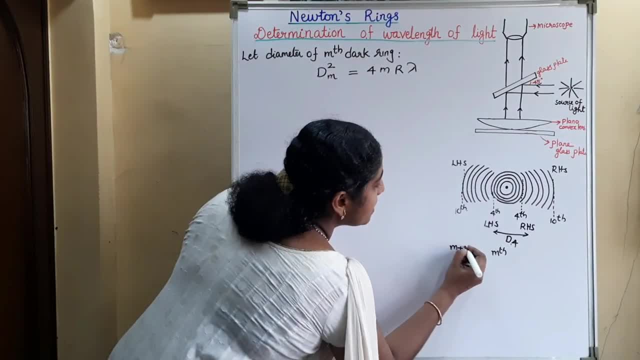 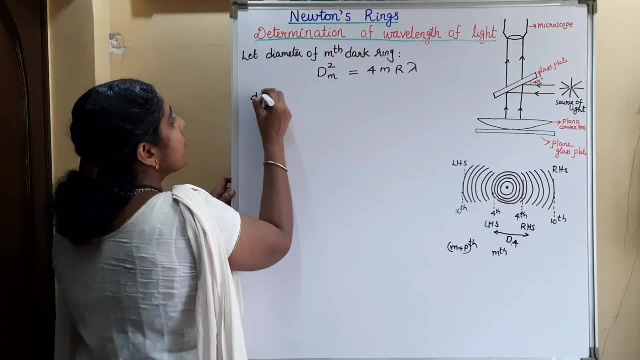 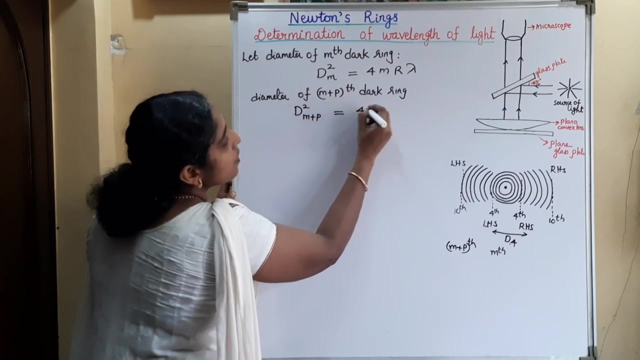 consider any other ring as the m plus pth dark ring. let be the m plus pth dark ring. then what will be the diameter of m plus pth darker ring? that is d square. m plus p is equal to 4 into m plus p r lambda, where p is the difference between the order of these two. 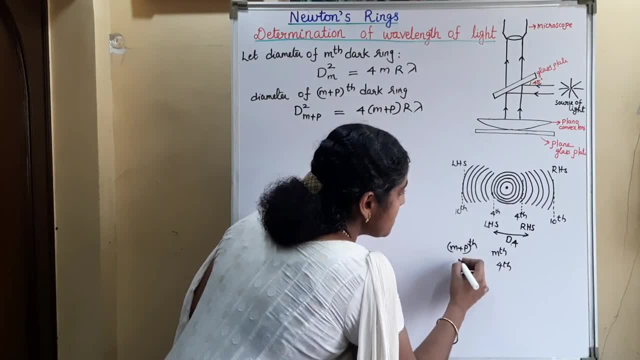 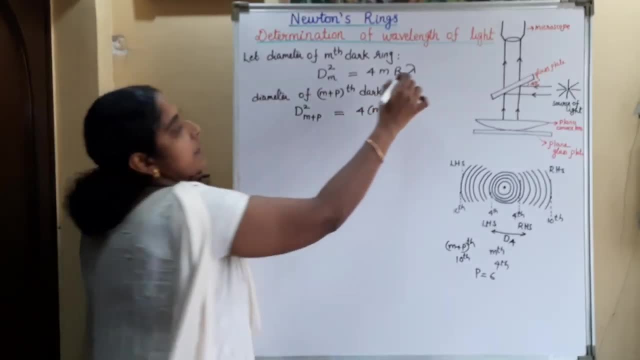 rings. here it is: mth ring is fourth and at m plus pth is a tenth ring. so this here p is equal to 10 minus 4, that is 6. so in general we can write the diameter of mth ring and m plus pth is equal to 4. 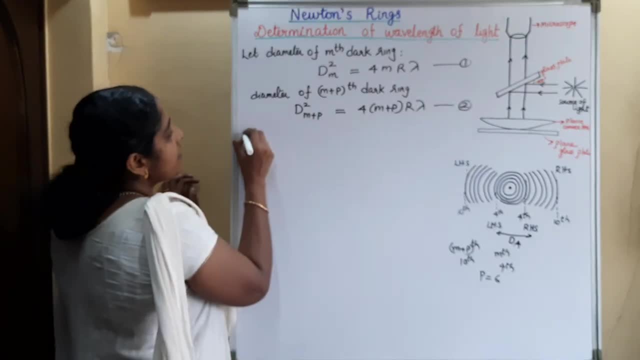 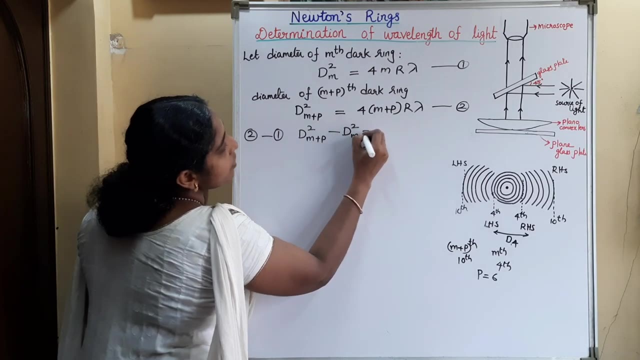 the darkening as in equation 1 and 2. then if you take the difference of equation 2 and 1, we will get d square m plus p minus d square m is equal to 4 m plus p r lambda minus 4 m r lambda. so we 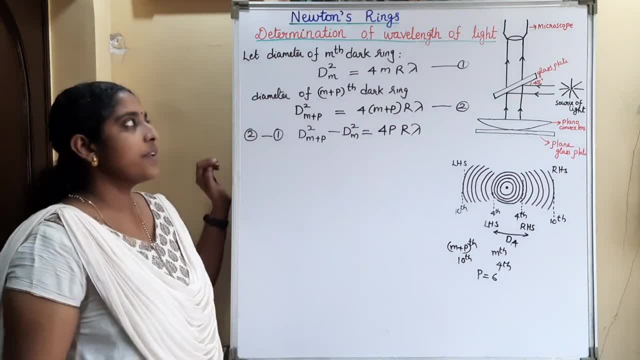 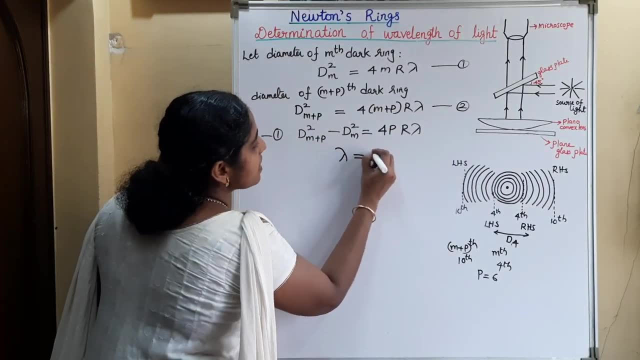 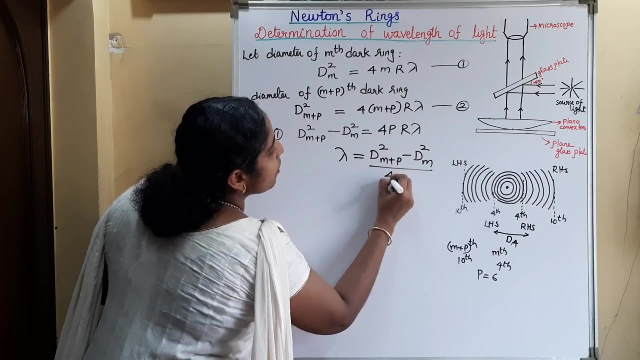 are getting 4 p r lambda what we want to find out if we want to find out the wavelength of light. so from this expression, what is the wavelength of light? lambda is equal to d square m plus p, minus d square m divided by 4 p? r. so this equation gives the wavelength of light. so in the 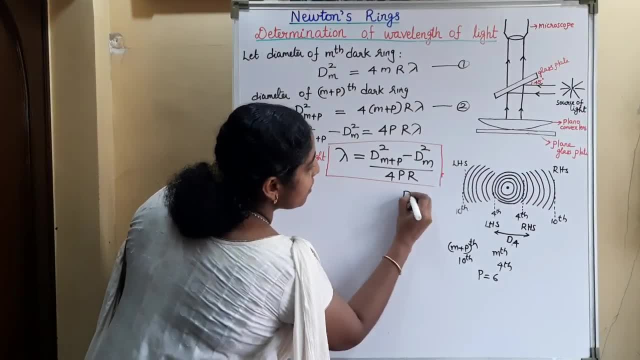 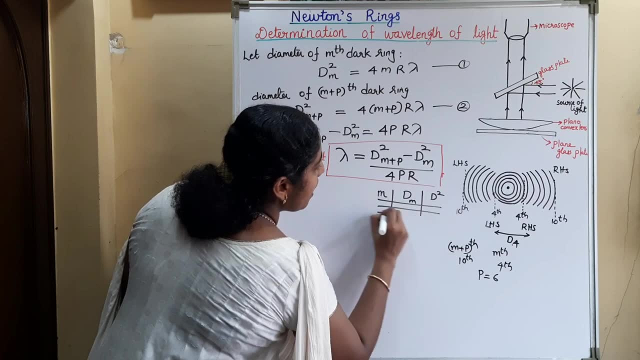 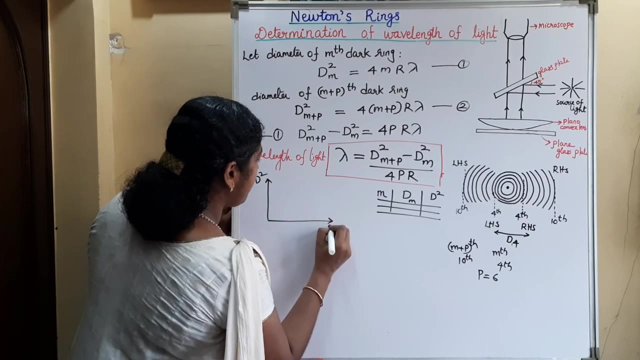 laboratory, while doing experiment, we can find out the diameter of various order. then we can find out the square of these diameters. then we can draw a graph of diameter square versus order. then we will get a straight line graph. then what will be the slope of this graph? 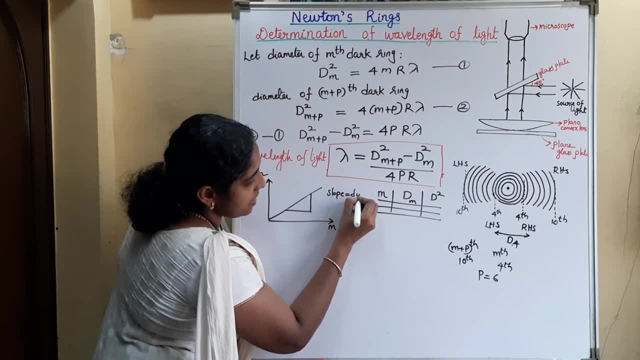 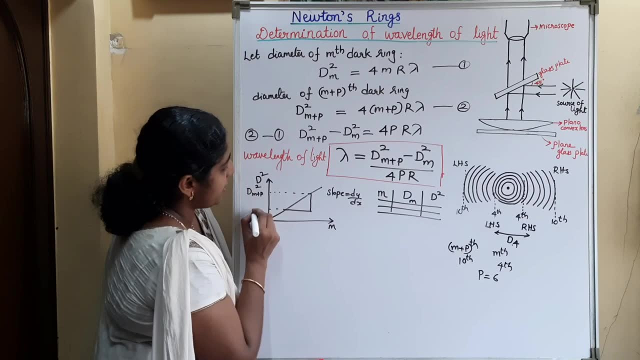 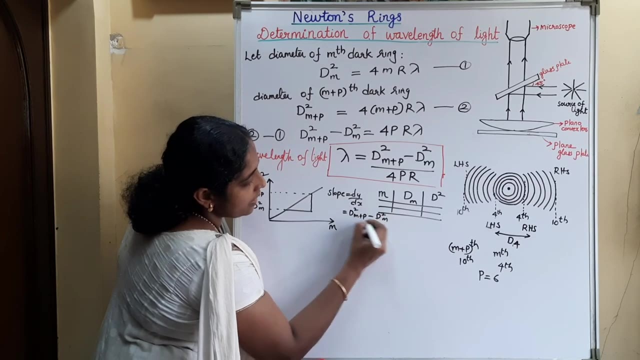 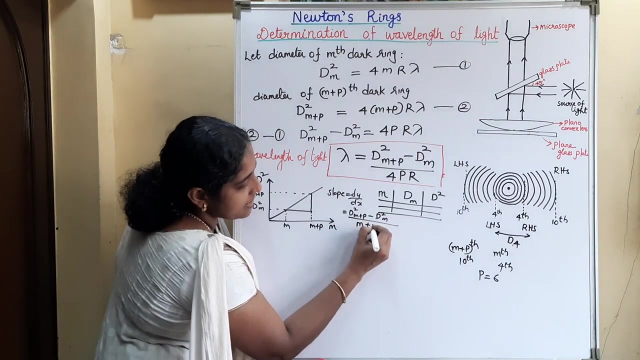 slope is equal to d y by d x. so this d y is diameter of m plus p square minus d square m. so d square m plus p minus d square m, divided by what will be this d x- that is this order- will be m plus p. this will be m. so this d x is m plus p minus m, so that is d square. 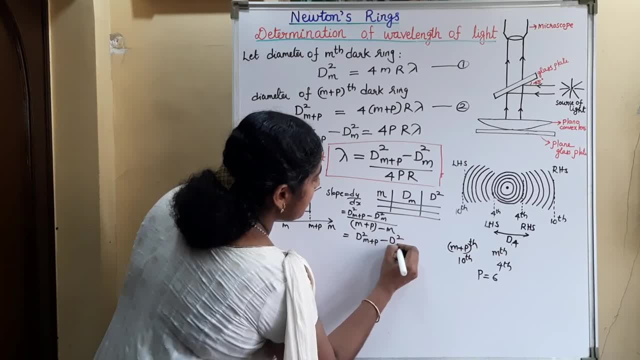 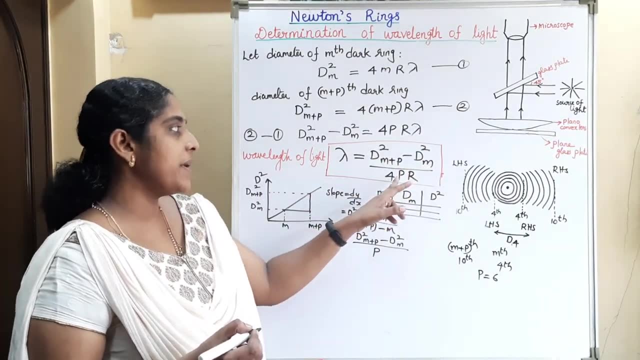 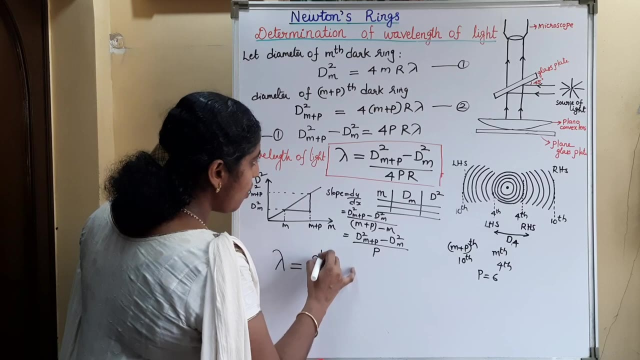 m plus p, minus d square m divided by p. so in this expression lambda is equal to d square m plus p, minus d square m divided by p. we can replace by this slope, so what will be the new expression for the wavelength of light? that is, slope divided by 4 r. so using this graph also, we can find out. 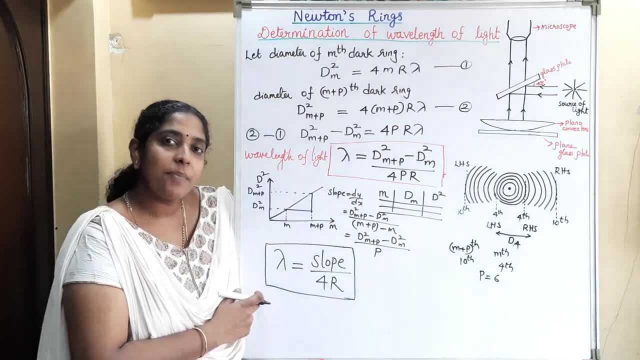 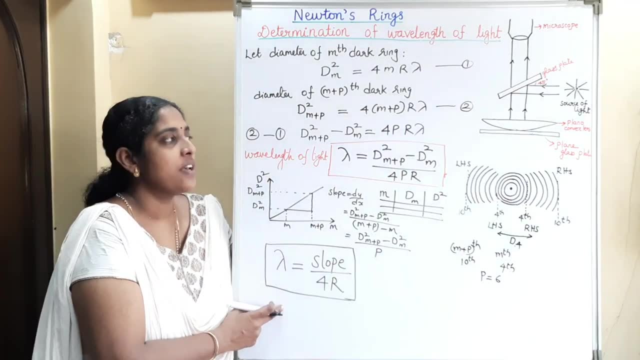 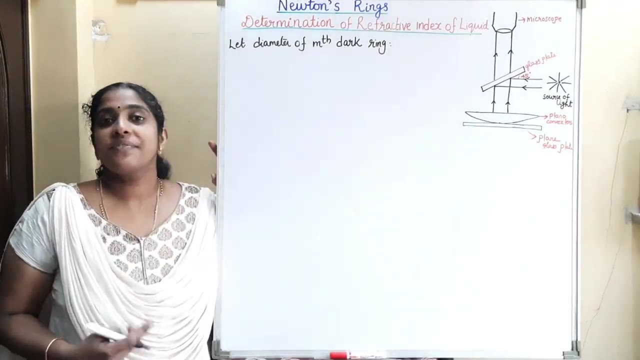 the wavelength of the light. another application of newton's ring is that if the wavelength is different, we can find out the radius of curvature also using these expressions. so these are the experimental arrangement for the determination of wavelength of light using newton's ring. next we can determine the refractive index of the liquid using newton's ring arrangement for that. 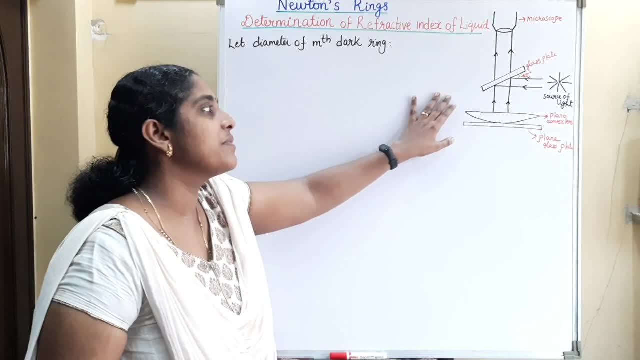 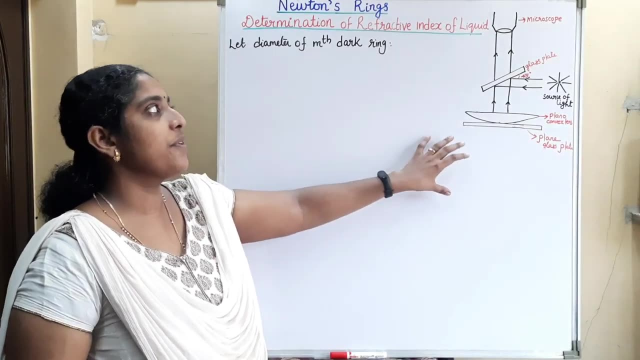 whose refractive index we have to determine that liquid is filled between the lens and the glass plate, and similar to that we discussed earlier. keep this set up before the microscope and the source of light. then the interference part will be determined and the resistance part will be. 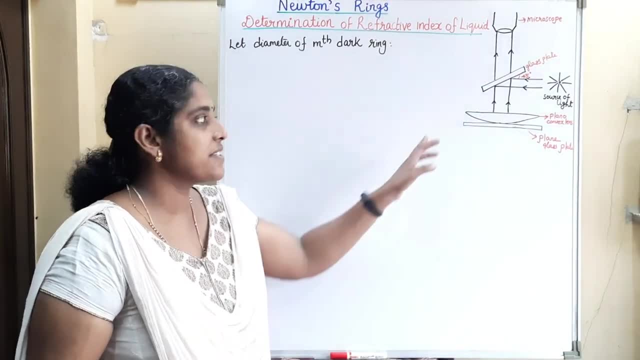 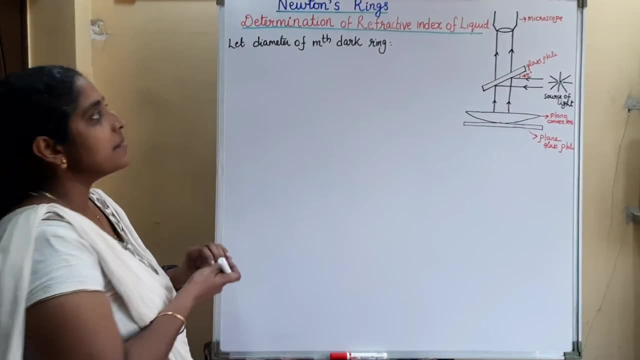 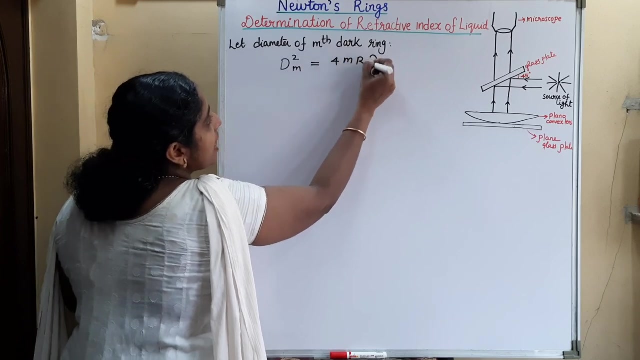 pattern is produced due to the superposition of the light reflected from the upper and bottom surface of the liquid film between this lens and the glass plate. Then diameter of mth dark ring is d square m is equal to 4 m r lambda divided by mu here, because here in between the lens and 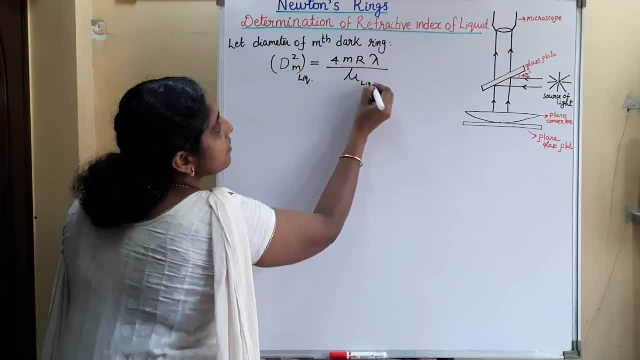 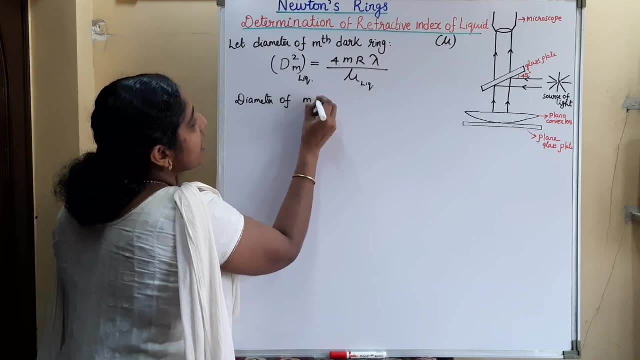 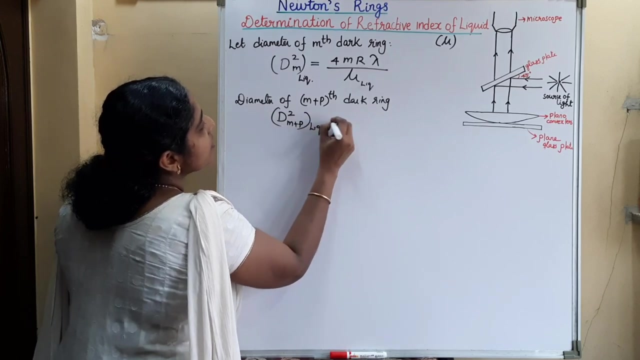 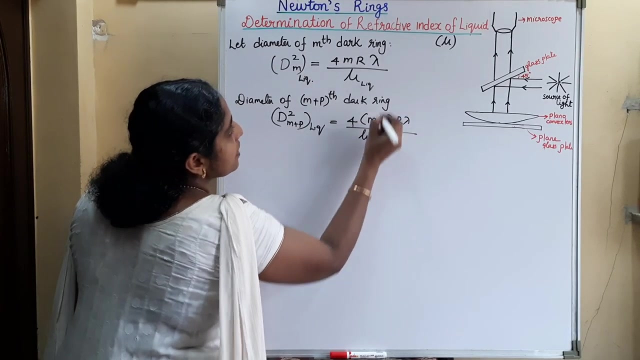 glass plate. there is a liquid. mu. here is the refractive index of the liquid. We can also write the diameter of m plus pth dark ring. that is equal to d square m plus p. liquid is equal to 4 into m plus p r lambda divided by mu. here mu is the refractive index of the liquid. This is: